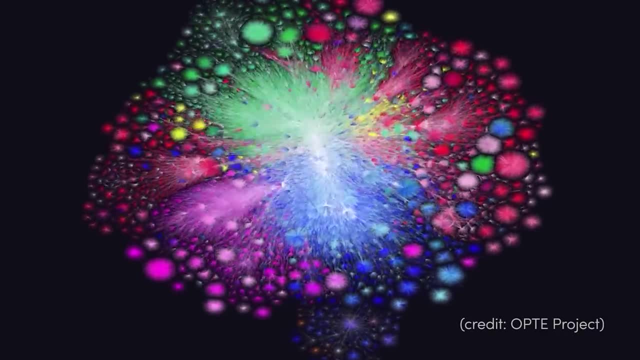 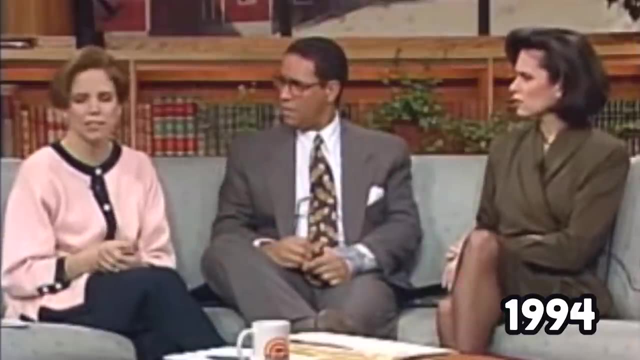 This is the internet. It's a network of billions of machines connected together. What do you write to it? like mail? No, a lot of people use it and communicate. I guess they can communicate with NBC writers and producers. Allison, can you explain what internet is? 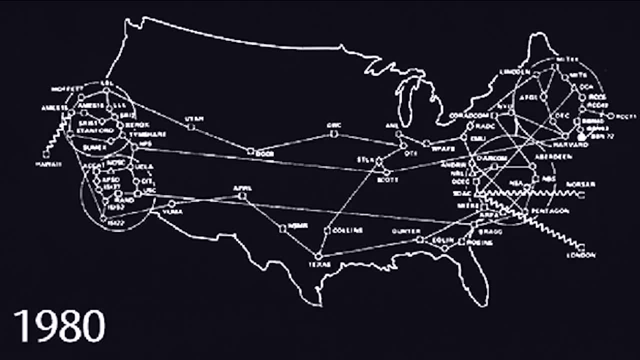 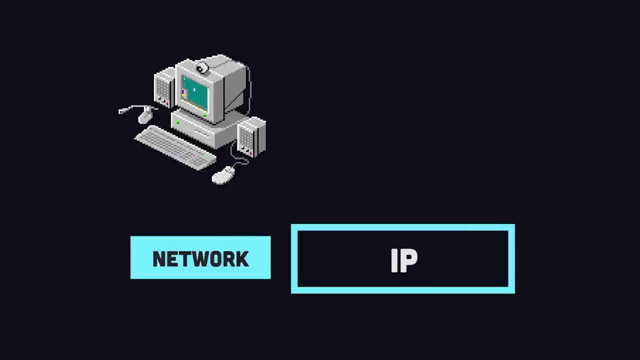 It was officially born on January 1st 1983, thanks to the establishment of the Internet Protocol Suite, which standardized the way these computers communicate. The Internet Protocol is used to identify different computers on the network by assigning each one of them a unique IP address. 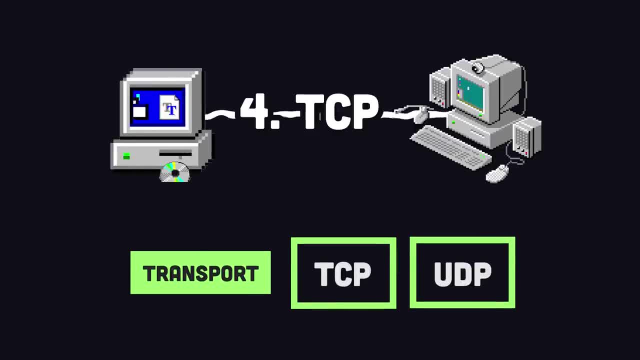 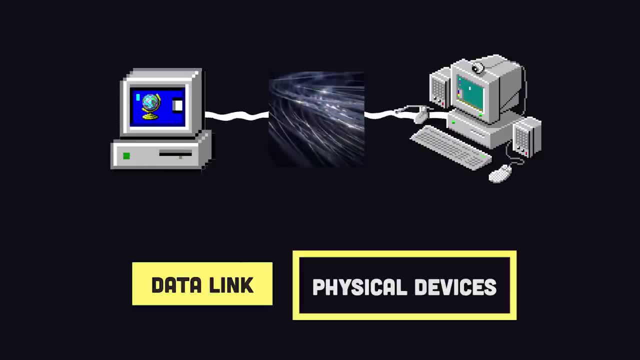 These computers can then send data back and forth. with the Transmission Control Protocol, It breaks data into a bunch of small packets, kind of like puzzle pieces, then sends them through a bunch of physical components like fiber optic cables and modems, before they're put back together by the receiving computer. 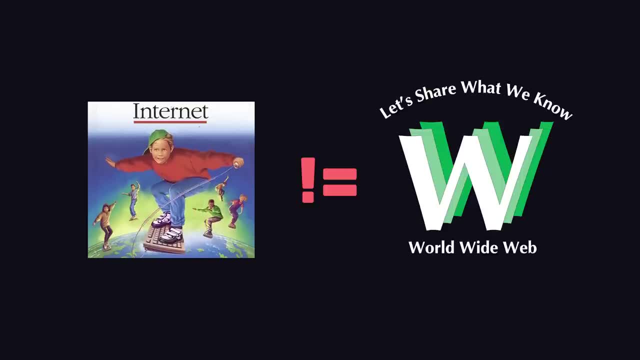 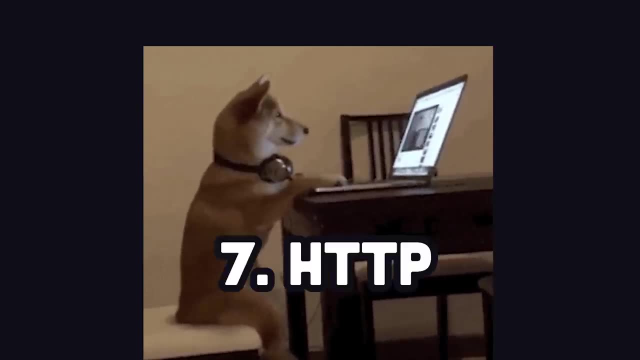 You can think of the internet as hardware, but the internet is not the same thing as the web. The World Wide Web is like software that sits on top of the internet, where people can access web pages with the Hypertext Transfer Protocol. What's special about it is that it gives every page of content a uniform resource. 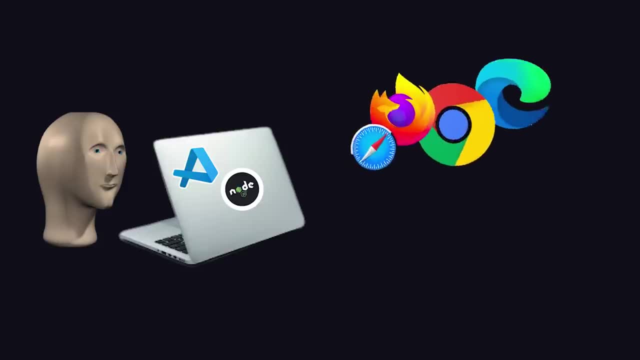 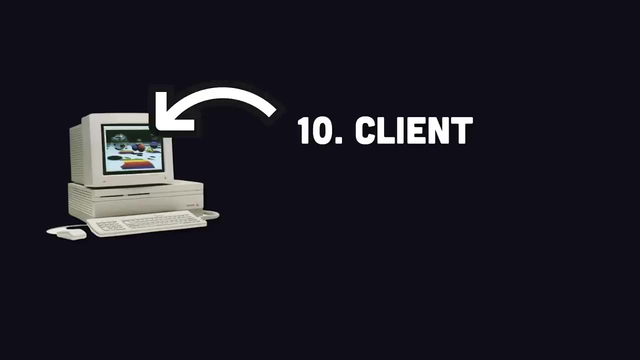 A resource locator or URL. Humans typically use a tool called a web browser to access a URL where it can be rendered visually on their screen. The browser is called the client because it's consuming information, but on the other end of that URL there's another computer called a server. 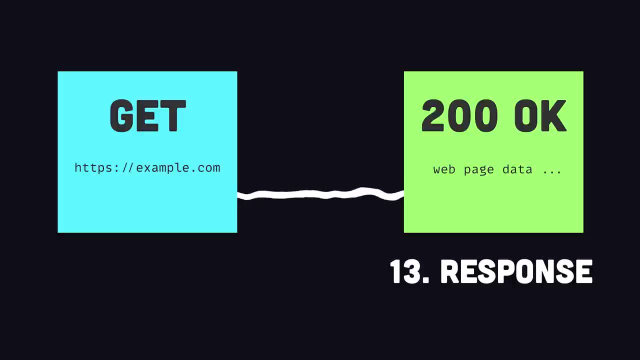 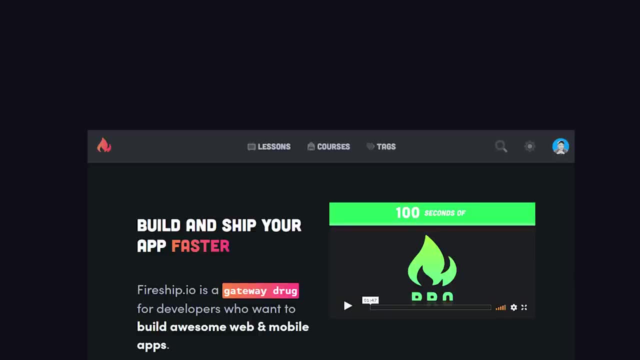 It received an HTTP request from the client, then sent a response containing the web page content. These are called HTTP messages, but more on that later. What's interesting is that every web page has a unique domain name, like fireshipio or examplecom. 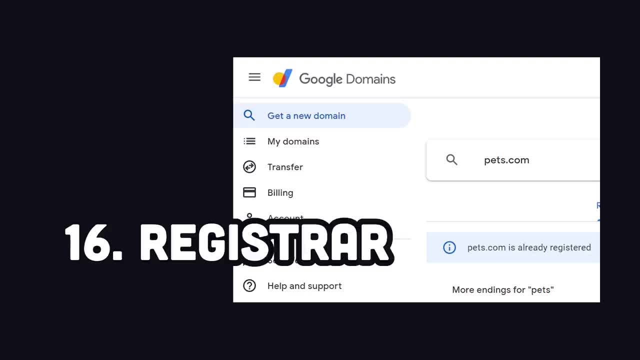 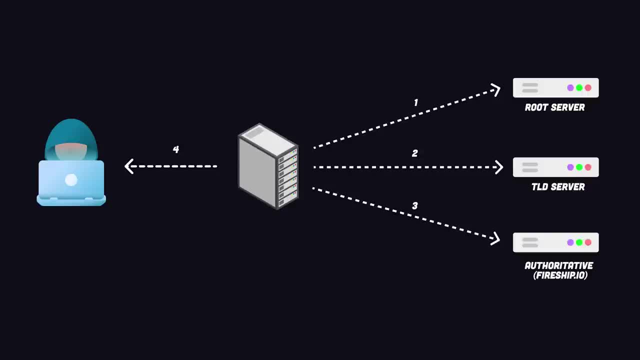 A domain name can be registered by anyone via a registrar who's accredited by ICANN, a non-profit responsible for overseeing namespaces on the internet. When you navigate to a domain in a browser, it gets routed through the domain name system that maps these names to an actual IP address on a server somewhere. 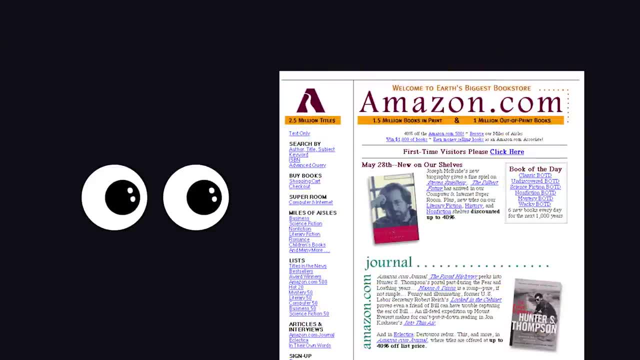 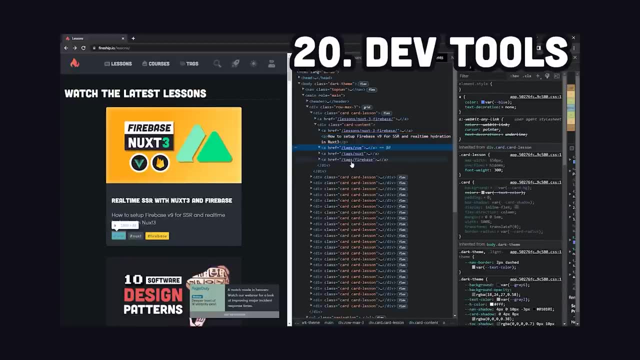 DNS is like the phone book of the internet. Now, when you look at a web page, the actual content you see is represented by hypertext markup language. Most browsers have dev tools where you can inspect the structure of the HTML at any time. 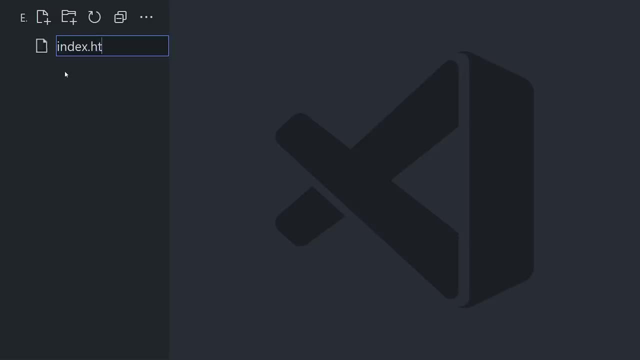 To build your own web page, you'll want a text library. You'll need a text editor like VSCode. An HTML document is just a collection of elements where an element is an opening and closing tag with some content in the middle like a paragraph and heading. 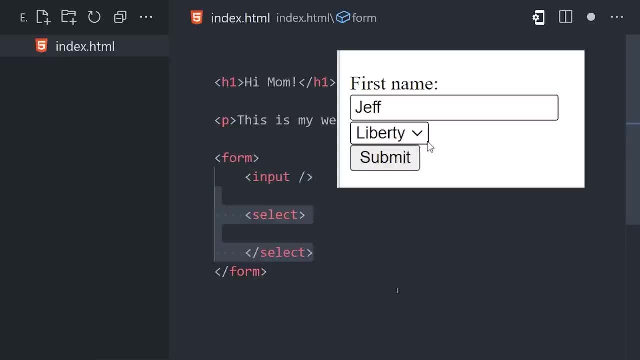 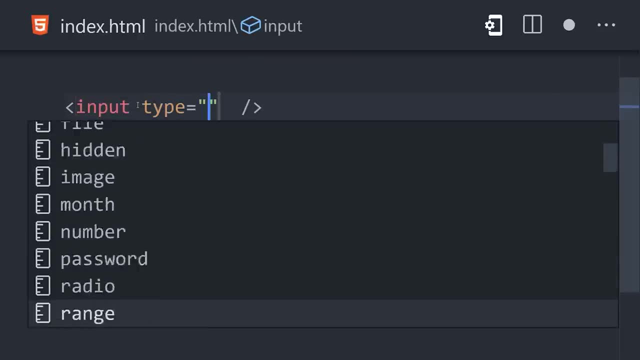 It also has elements that handle user input, like the select and input elements, which are used to build forms. In addition, elements can have one or more attributes to change their behavior. For example, an input can have a type like text or number, which the browser will render differently to collect the appropriate value. 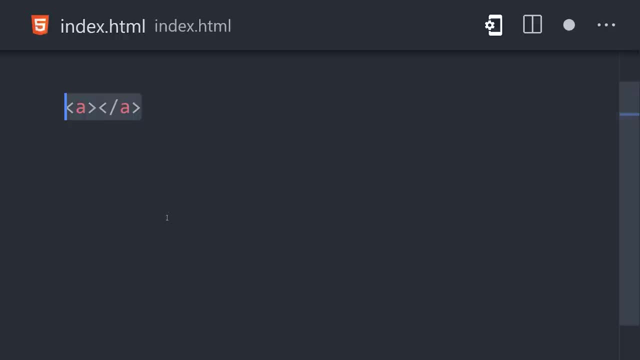 But the element that puts the hypertext in HTML is the A tag, which is the type of text the browser will render differently to collect the appropriate value. But the element that puts the hypertext in HTML is the A tag, which is the type of text in HTML. 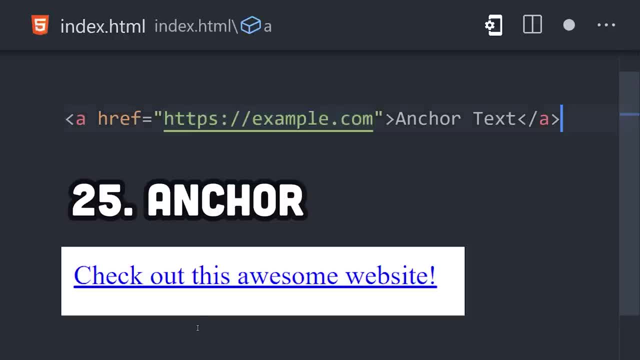 It's a link that allows one page to navigate to a different page based on its URL. It's a link that allows one page to navigate to a different page based on its URL. It's a link that allows one page to navigate to a different page based on its URL. 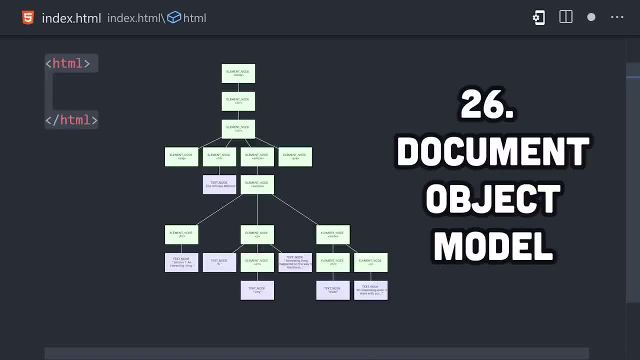 These elements are nested together in a hierarchy to form the Document Object, Model or DOM. These elements are nested together in a hierarchy to form the Document Object, Model or DOM. From the root element, a web page is split into two parts. From the root element, a web page is split into two parts. 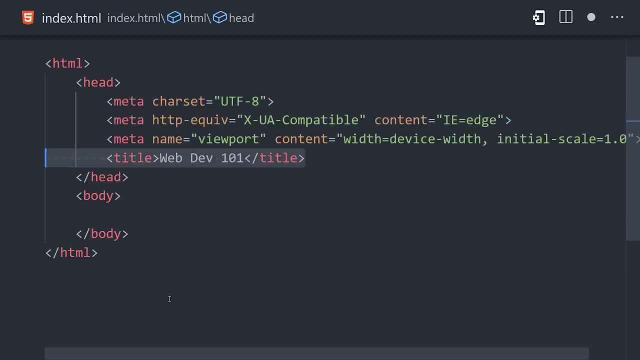 The head contains invisible content like metadata and a title. Then we have the body for the main content that the end user actually sees. Then we have the body for the main content that the end user actually sees. The reason we wrap everything in tags is to give browsers and bots hints about the semantic meaning of the web page. 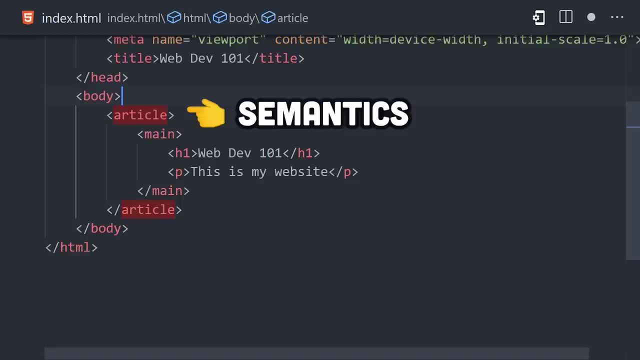 The reason we wrap everything in tags is to give browsers and bots hints about the semantic meaning of the web page. The reason we wrap everything in tags is to give browsers and bots hints about the semantic meaning of the web page. This allows search engines to display results properly and also helps with accessibility for devices like screen readers that allow anybody, regardless of disability, to enjoy the content. 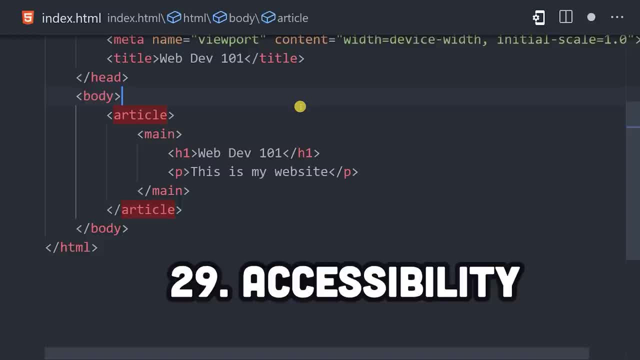 This allows search engines to display results properly and also helps with accessibility for devices like screen readers that allow anybody, regardless of disability, to enjoy the content. This allows search engines to display results properly and also helps with accessibility for devices like screen readers that allow anybody, regardless of disability, to enjoy the content. 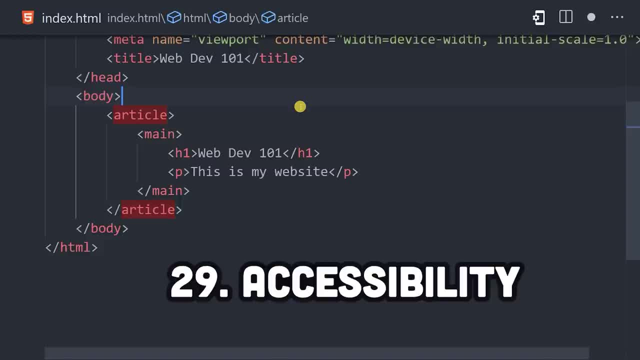 This allows search engines to display results properly and also helps with accessibility for devices like screen readers that allow anybody, regardless of disability, to enjoy the content. This allows search engines to display results properly and also helps with accessibility for devices like screen readers that allow anybody, regardless of disability, to enjoy the content. 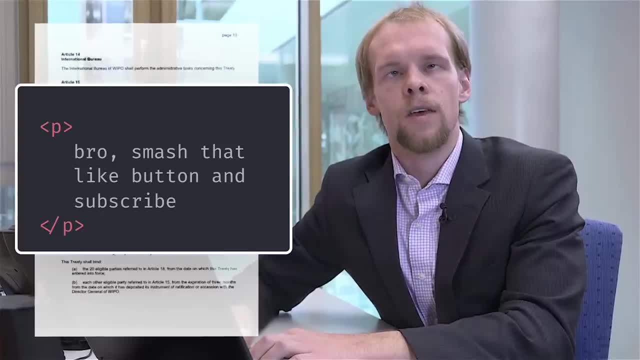 This allows search engines to display results properly and also helps with accessibility for devices like screen readers that allow anybody, regardless of disability, to enjoy the content. This allows search engines to display results properly and also helps with accessibility for devices like screen readers that allow anybody, regardless of disability, to enjoy the content. 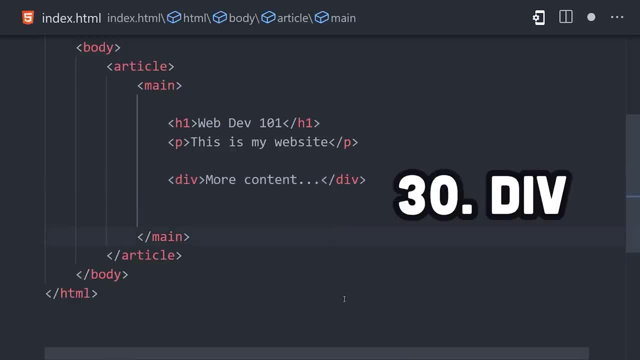 This allows search engines to display results properly and also helps with accessibility for devices like screen readers that allow anybody, regardless of disability, to enjoy the content. This allows search engines to display results properly and also helps with accessibility for devices like screen readers that allow anybody, regardless of disability, to enjoy the content. 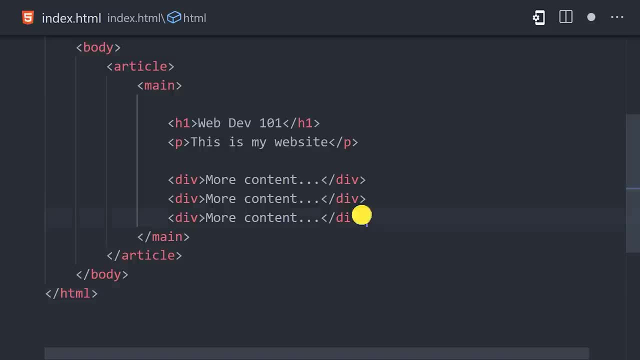 This allows search engines to display results properly and also helps with accessibility for devices like screen readers that allow anybody, regardless of disability, to enjoy the content. This allows search engines to display results properly and also helps with accessibility for devices like screen readers that allow anybody, regardless of disability, to enjoy the content. 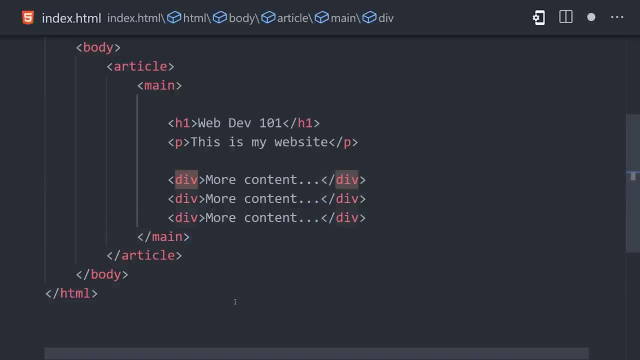 This allows search engines to display results properly and also helps with accessibility for devices like screen readers that allow anybody, regardless of disability, to enjoy the content. This allows search engines to display results properly and also helps with accessibility for devices like screen readers that allow anybody, regardless of disability, to enjoy the content. 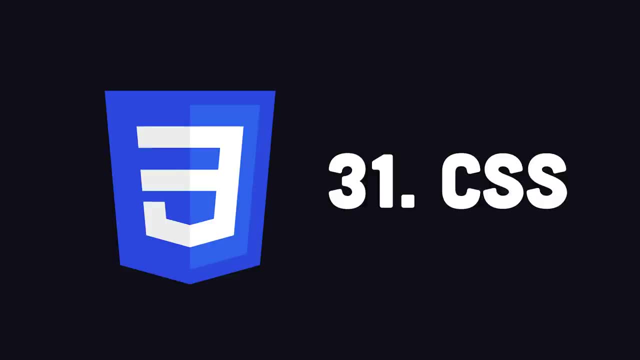 This allows search engines to display results properly and also helps with accessibility for devices like screen readers that allow anybody, regardless of disability, to enjoy the content. This allows search engines to display results properly and also helps with accessibility for devices like screen readers that allow anybody, regardless of disability, to enjoy the content. 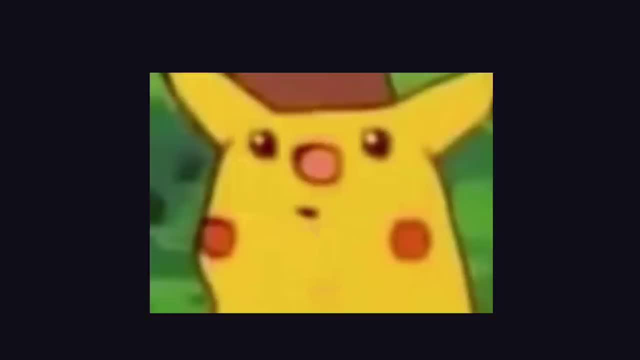 This allows search engines to display results properly and also helps with accessibility for devices like screen readers that allow anybody, regardless of disability, to enjoy the content. This allows search engines to display results properly and also helps with accessibility for devices like screen readers that allow anybody, regardless of disability, to enjoy the content. 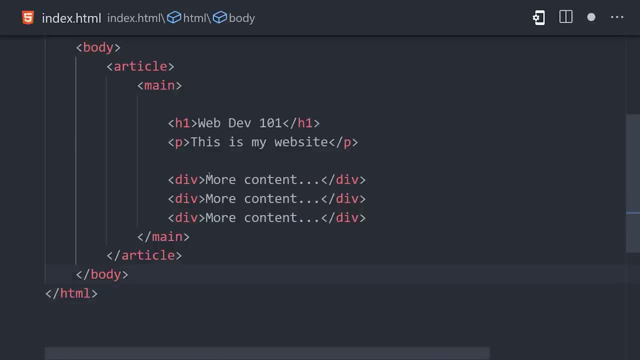 This allows search engines to display results properly and also helps with accessibility for devices like screen readers that allow anybody, regardless of disability, to enjoy the content. This allows search engines to display results properly and also helps with accessibility for devices like screen readers that allow anybody, regardless of disability, to enjoy the content. 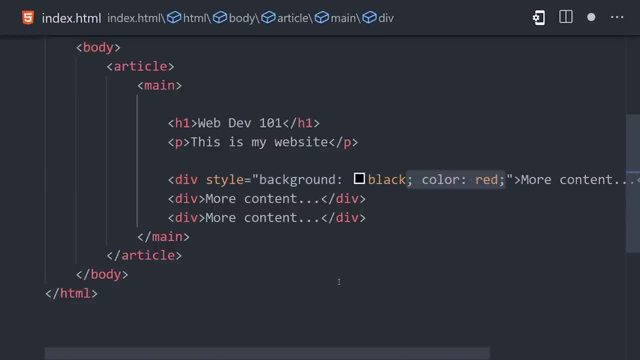 This allows search engines to display results properly and also helps with accessibility for devices like screen readers that allow anybody, regardless of disability, to enjoy the content. This allows search engines to display results properly and also helps with accessibility for devices like screen readers that allow anybody, regardless of disability, to enjoy the content. 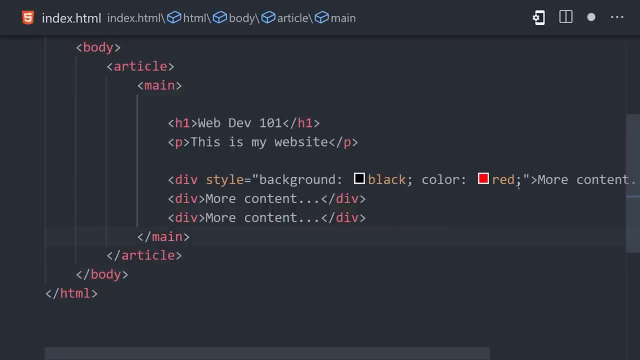 This allows search engines to display results properly and also helps with accessibility for devices like screen readers that allow anybody, regardless of disability, to enjoy the content. This allows search engines to display results properly and also helps with accessibility for devices like screen readers that allow anybody, regardless of disability, to enjoy the content. 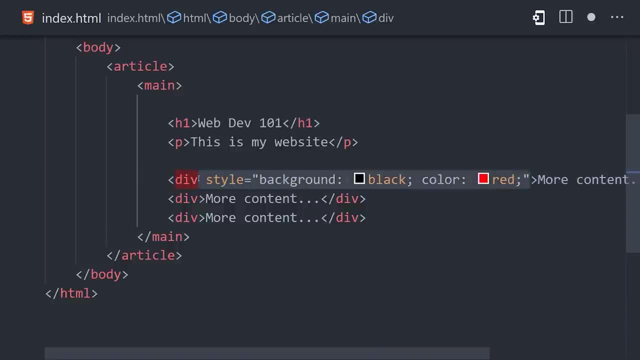 This allows search engines to display results properly and also helps with accessibility for devices like screen readers that allow anybody, regardless of disability, to enjoy the content. This allows search engines to display results properly and also helps with accessibility for devices like screen readers that allow anybody, regardless of disability, to enjoy the content. 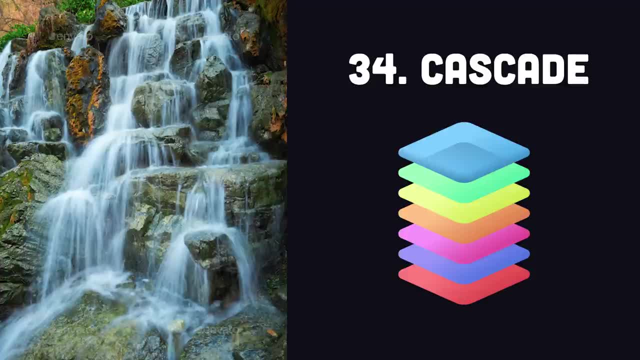 This allows search engines to display results properly and also helps with accessibility for devices like screen readers that allow anybody, regardless of disability, to enjoy the content. This allows search engines to display results properly and also helps with accessibility for devices like screen readers that allow anybody, regardless of disability, to enjoy the content. 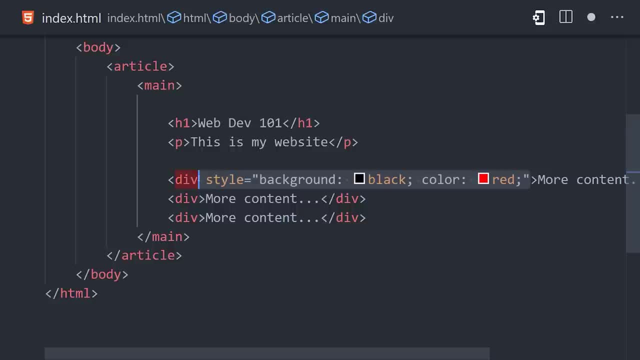 This allows search engines to display results properly and also helps with accessibility for devices like screen readers that allow anybody, regardless of disability, to enjoy the content. This allows search engines to display results properly and also helps with accessibility for devices like screen readers that allow anybody, regardless of disability, to enjoy the content. 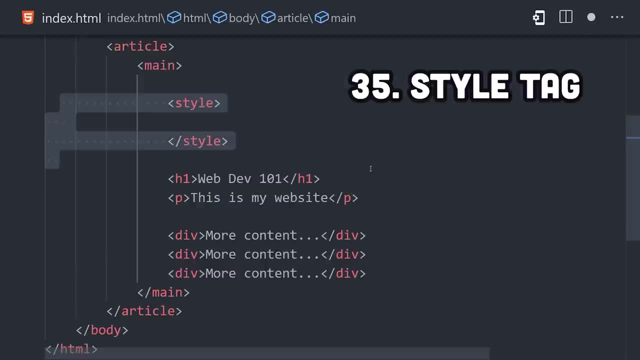 This allows search engines to display results properly and also helps with accessibility for devices like screen readers that allow anybody, regardless of disability, to enjoy the content. This allows search engines to display results properly and also helps with accessibility for devices like screen readers that allow anybody, regardless of disability, to enjoy the content. 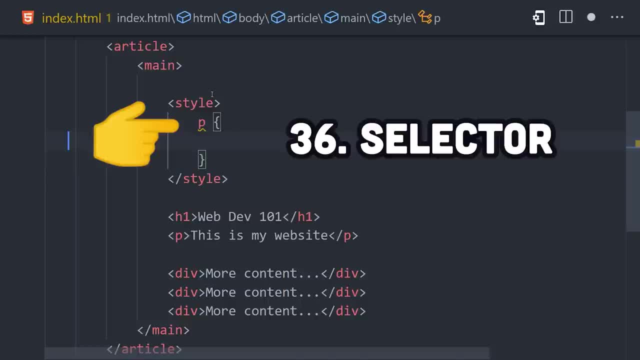 This allows search engines to display results properly and also helps with accessibility for devices like screen readers that allow anybody, regardless of disability, to enjoy the content. This allows search engines to display results properly and also helps with accessibility for devices like screen readers that allow anybody, regardless of disability, to enjoy the content. 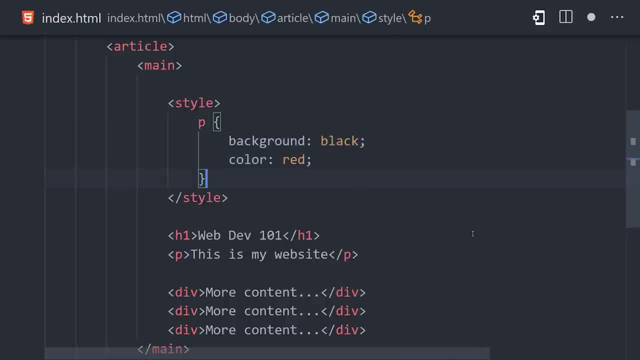 This allows search engines to display results properly and also helps with accessibility for devices like screen readers that allow anybody, regardless of disability, to enjoy the content. This allows search engines to display results properly and also helps with accessibility for devices like screen readers that allow anybody, regardless of disability, to enjoy the content. 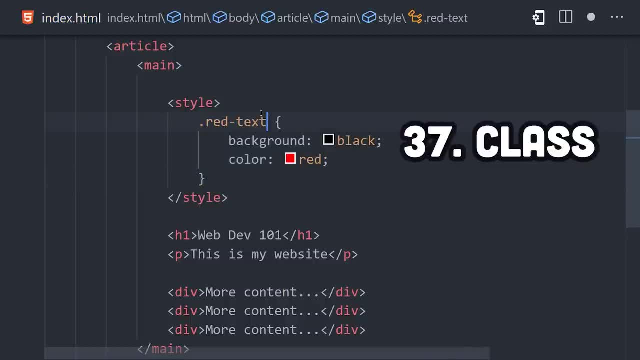 This allows search engines to display results properly and also helps with accessibility for devices like screen readers that allow anybody, regardless of disability, to enjoy the content. This allows search engines to display results properly and also helps with accessibility for devices like screen readers that allow anybody, regardless of disability, to enjoy the content. 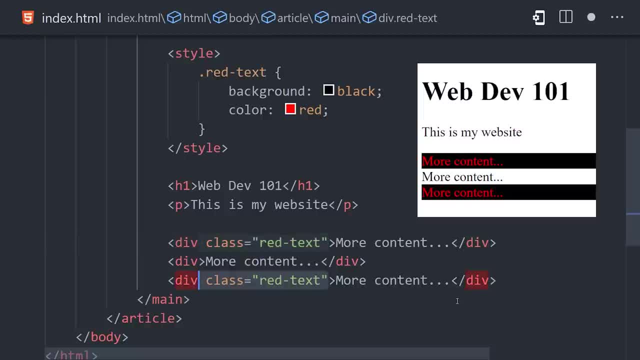 This allows search engines to display results properly and also helps with accessibility for devices like screen readers that allow anybody, regardless of disability, to enjoy the content. This allows search engines to display results properly and also helps with accessibility for devices like screen readers that allow anybody, regardless of disability, to enjoy the content. 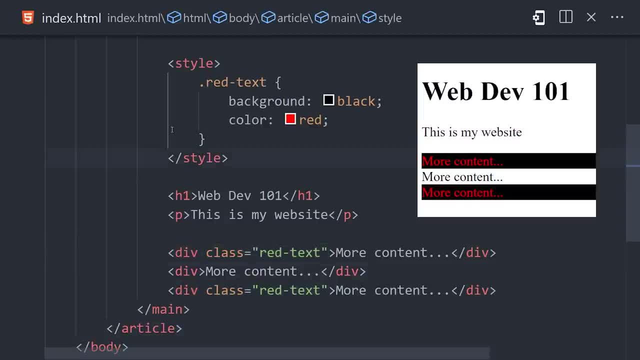 This allows search engines to display results properly and also helps with accessibility for devices like screen readers that allow anybody, regardless of disability, to enjoy the content. This allows search engines to display results properly and also helps with accessibility for devices like screen readers that allow anybody, regardless of disability, to enjoy the content. 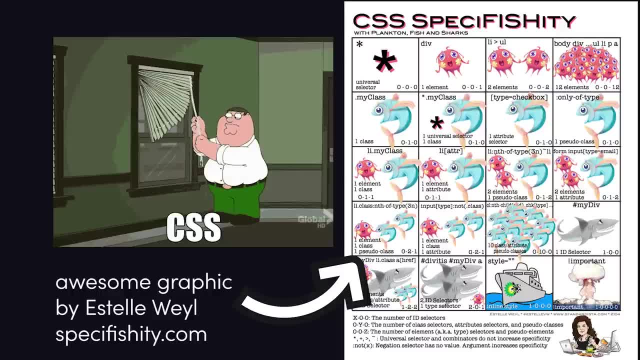 This allows search engines to display results properly and also helps with accessibility for devices like screen readers that allow anybody, regardless of disability, to enjoy the content. This allows search engines to display results properly and also helps with accessibility for devices like screen readers that allow anybody, regardless of disability, to enjoy the content. 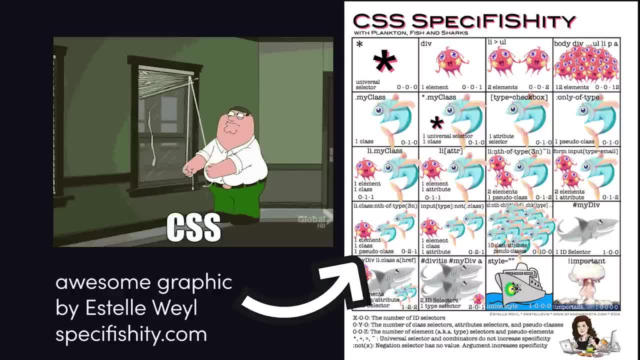 This allows search engines to display results properly and also helps with accessibility for devices like screen readers that allow anybody, regardless of disability, to enjoy the content. This allows search engines to display results properly and also helps with accessibility for devices like screen readers that allow anybody, regardless of disability, to enjoy the content. 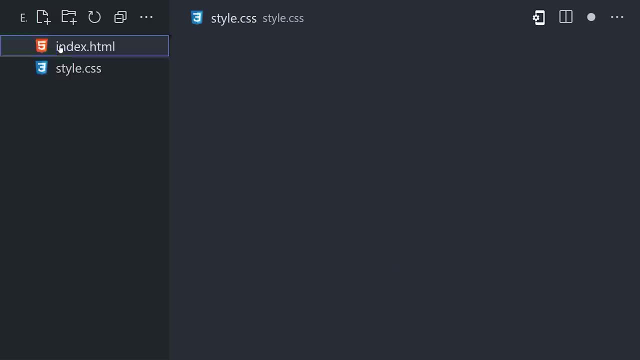 This allows search engines to display results properly and also helps with accessibility for devices like screen readers that allow anybody, regardless of disability, to enjoy the content. This allows search engines to display results properly and also helps with accessibility for devices like screen readers that allow anybody, regardless of disability, to enjoy the content. 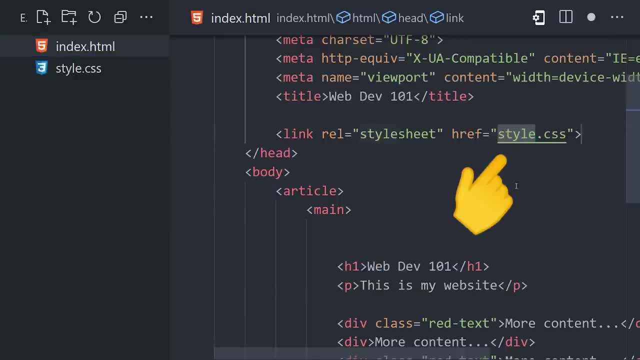 This allows search engines to display results properly and also helps with accessibility for devices like screen readers that allow anybody, regardless of disability, to enjoy the content. This allows search engines to display results properly and also helps with accessibility for devices like screen readers that allow anybody, regardless of disability, to enjoy the content. 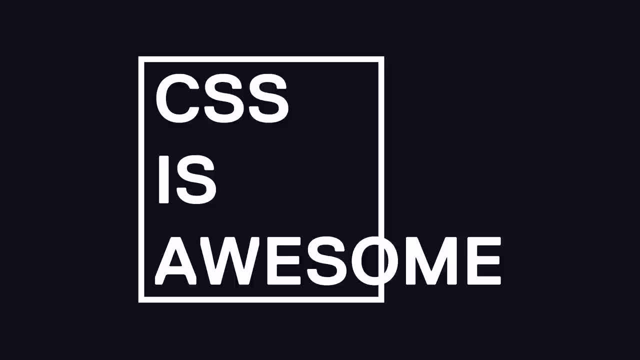 This allows search engines to display results properly and also helps with accessibility for devices like screen readers that allow anybody, regardless of disability, to enjoy the content. This allows search engines to display results properly and also helps with accessibility for devices like screen readers that allow anybody, regardless of disability, to enjoy the content. 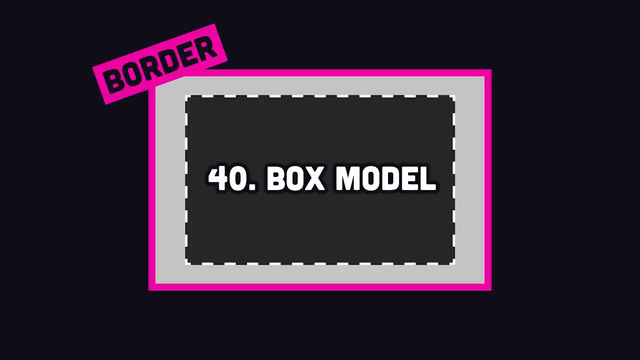 This allows search engines to display results properly and also helps with accessibility for devices like screen readers that allow anybody, regardless of disability, to enjoy the content. This allows search engines to display results properly and also helps with accessibility for devices like screen readers that allow anybody, regardless of disability, to enjoy the content. 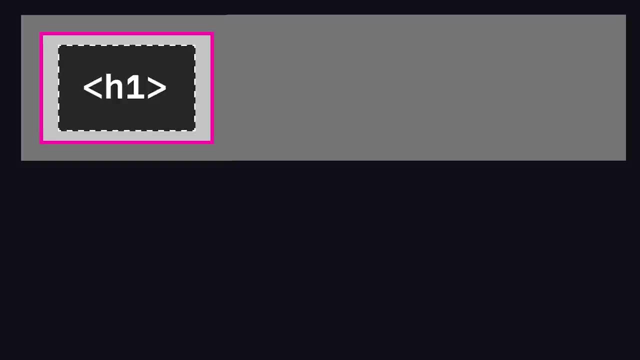 This allows search engines to display results properly and also helps with accessibility for devices like screen readers that allow anybody, regardless of disability, to enjoy the content. This allows search engines to display results properly and also helps with accessibility for devices like screen readers that allow anybody, regardless of disability, to enjoy the content. 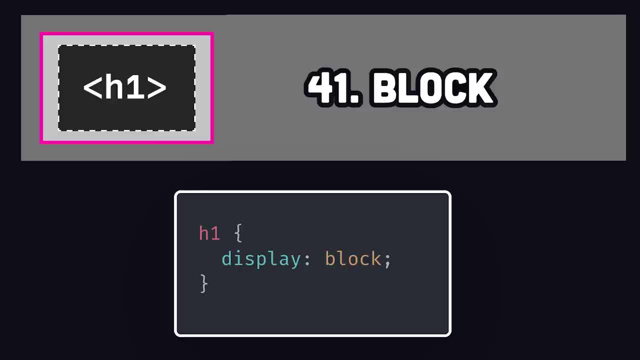 This allows search engines to display results properly and also helps with accessibility for devices like screen readers that allow anybody, regardless of disability, to enjoy the content. This allows search engines to display results properly and also helps with accessibility for devices like screen readers that allow anybody, regardless of disability, to enjoy the content. 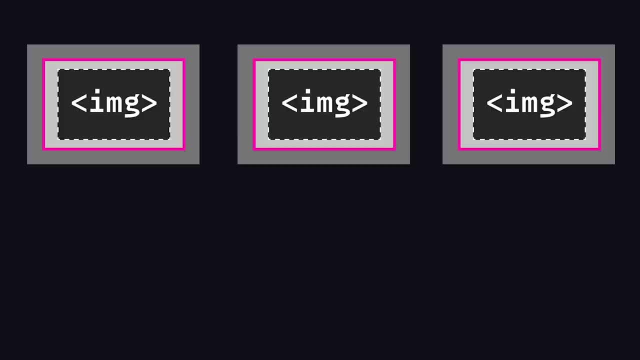 This allows search engines to display results properly and also helps with accessibility for devices like screen readers that allow anybody, regardless of disability, to enjoy the content. This allows search engines to display results properly and also helps with accessibility for devices like screen readers that allow anybody, regardless of disability, to enjoy the content. 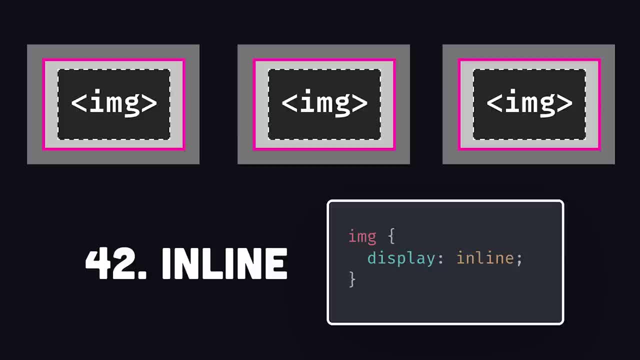 This allows search engines to display results properly and also helps with accessibility for devices like screen readers that allow anybody, regardless of disability, to enjoy the content. This allows search engines to display results properly and also helps with accessibility for devices like screen readers that allow anybody, regardless of disability, to enjoy the content. 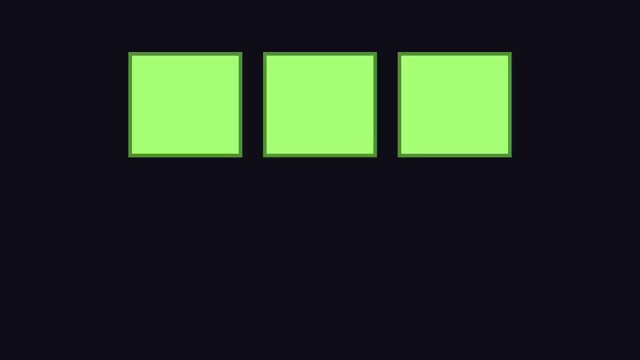 This allows search engines to display results properly and also helps with accessibility for devices like screen readers that allow anybody, regardless of disability, to enjoy the content. This allows search engines to display results properly and also helps with accessibility for devices like screen readers that allow anybody, regardless of disability, to enjoy the content. 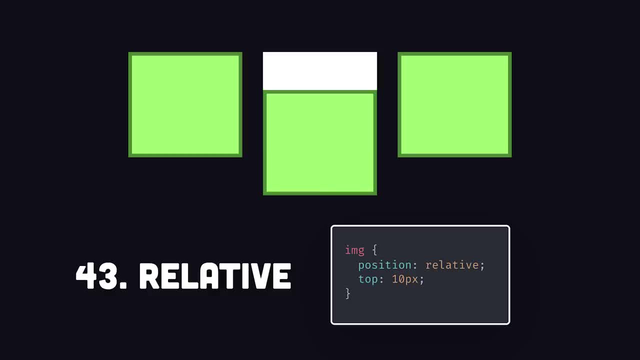 This allows search engines to display results properly and also helps with accessibility for devices like screen readers that allow anybody, regardless of disability, to enjoy the content. This allows search engines to display results properly and also helps with accessibility for devices like screen readers that allow anybody, regardless of disability, to enjoy the content. 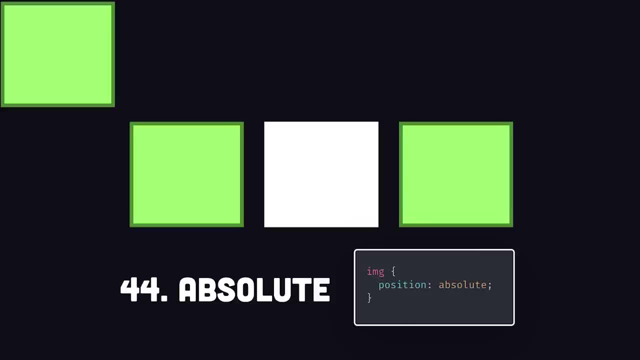 This allows search engines to display results properly and also helps with accessibility for devices like screen readers that allow anybody, regardless of disability, to enjoy the content. This allows search engines to display results properly and also helps with accessibility for devices like screen readers that allow anybody, regardless of disability, to enjoy the content. 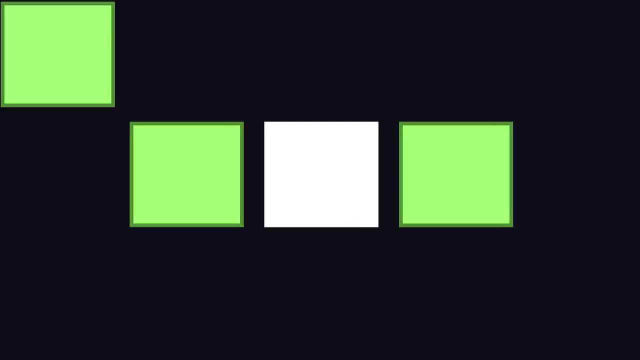 This allows search engines to display results properly and also helps with accessibility for devices like screen readers that allow anybody, regardless of disability, to enjoy the content. This allows search engines to display results properly and also helps with accessibility for devices like screen readers that allow anybody, regardless of disability, to enjoy the content. 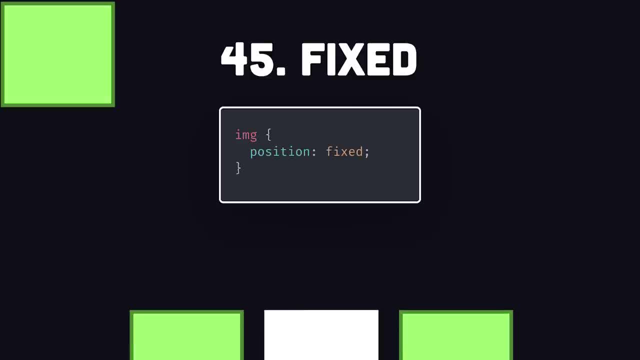 This allows search engines to display results properly and also helps with accessibility for devices like screen readers that allow anybody, regardless of disability, to enjoy the content. This allows search engines to display results properly and also helps with accessibility for devices like screen readers that allow anybody, regardless of disability, to enjoy the content. 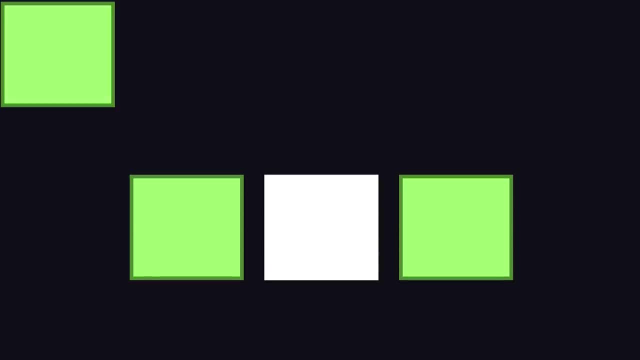 This allows search engines to display results properly and also helps with accessibility for devices like screen readers that allow anybody, regardless of disability, to enjoy the content. This allows search engines to display results properly and also helps with accessibility for devices like screen readers that allow anybody, regardless of disability, to enjoy the content. 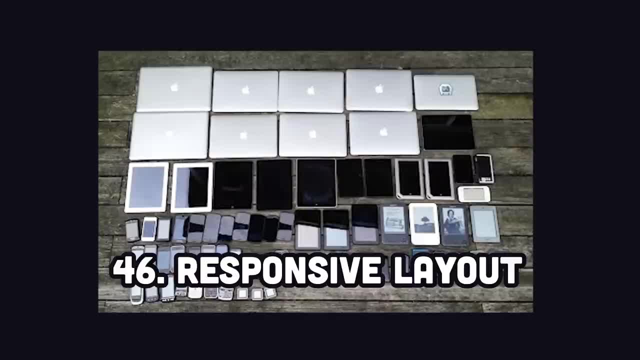 This allows search engines to display results properly and also helps with accessibility for devices like screen readers that allow anybody, regardless of disability, to enjoy the content. This allows search engines to display results properly and also helps with accessibility for devices like screen readers that allow anybody, regardless of disability, to enjoy the content. 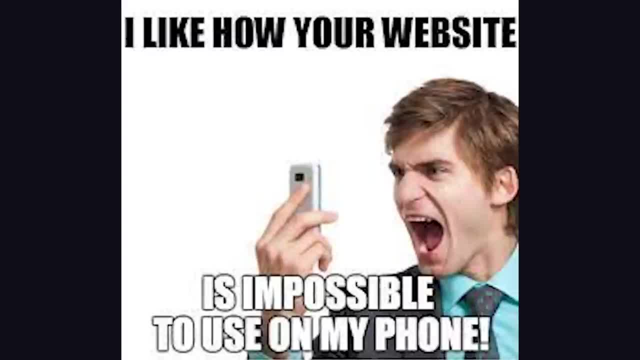 This allows search engines to display results properly and also helps with accessibility for devices like screen readers that allow anybody, regardless of disability, to enjoy the content. This allows search engines to display results properly and also helps with accessibility for devices like screen readers that allow anybody, regardless of disability, to enjoy the content. 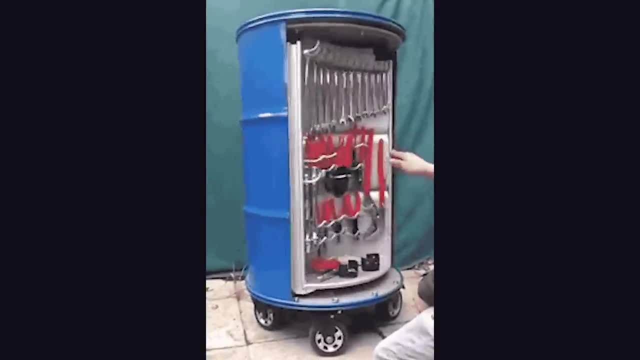 This allows search engines to display results properly and also helps with accessibility for devices like screen readers that allow anybody, regardless of disability, to enjoy the content. This allows search engines to display results properly and also helps with accessibility for devices like screen readers that allow anybody, regardless of disability, to enjoy the content. 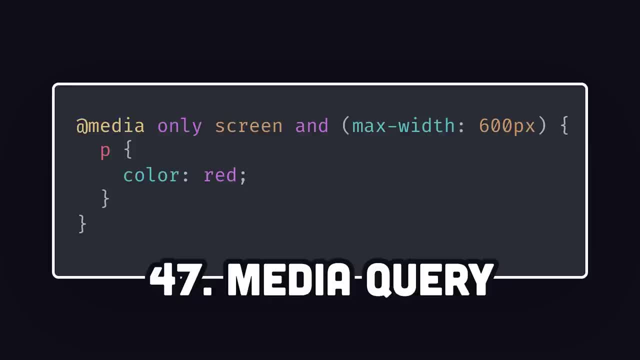 This allows search engines to display results properly and also helps with accessibility for devices like screen readers that allow anybody, regardless of disability, to enjoy the content. This allows search engines to display results properly and also helps with accessibility for devices like screen readers that allow anybody, regardless of disability, to enjoy the content. 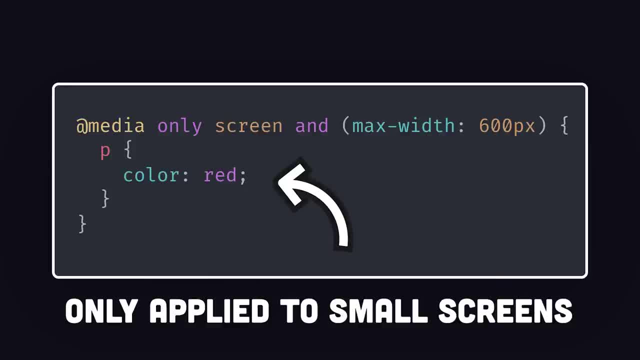 This allows search engines to display results properly and also helps with accessibility for devices like screen readers that allow anybody, regardless of disability, to enjoy the content. This allows search engines to display results properly and also helps with accessibility for devices like screen readers that allow anybody, regardless of disability, to enjoy the content. 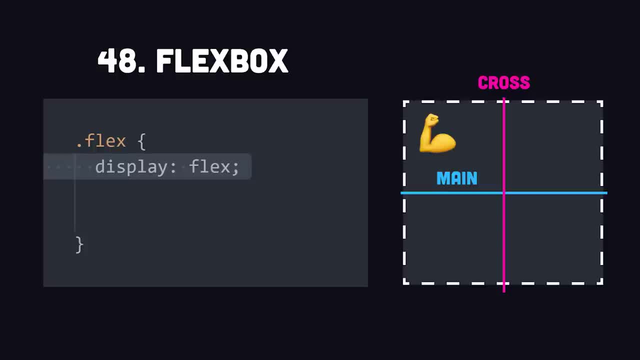 This allows search engines to display results properly and also helps with accessibility for devices like screen readers that allow anybody, regardless of disability, to enjoy the content. This allows search engines to display results properly and also helps with accessibility for devices like screen readers that allow anybody, regardless of disability, to enjoy the content. 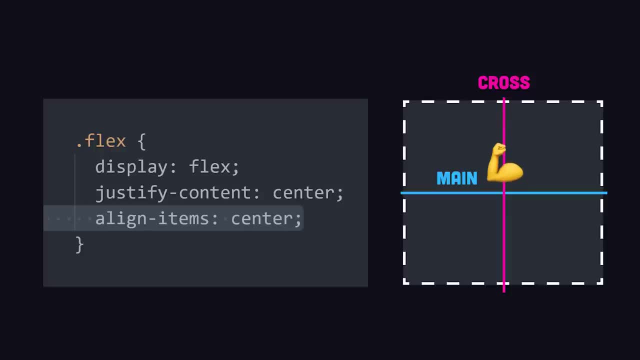 This allows search engines to display results properly and also helps with accessibility for devices like screen readers that allow anybody, regardless of disability, to enjoy the content. This allows search engines to display results properly and also helps with accessibility for devices like screen readers that allow anybody, regardless of disability, to enjoy the content. 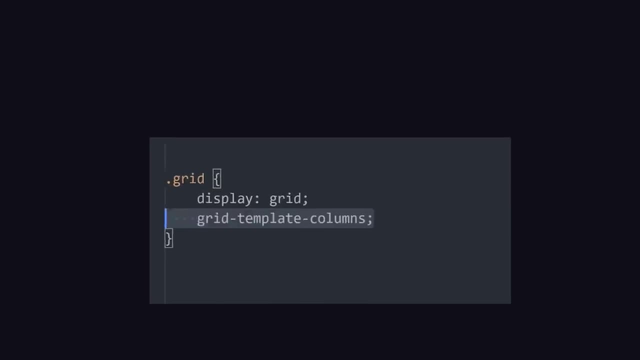 This allows search engines to display results properly and also helps with accessibility for devices like screen readers that allow anybody, regardless of disability, to enjoy the content. This allows search engines to display results properly and also helps with accessibility for devices like screen readers that allow anybody, regardless of disability, to enjoy the content. 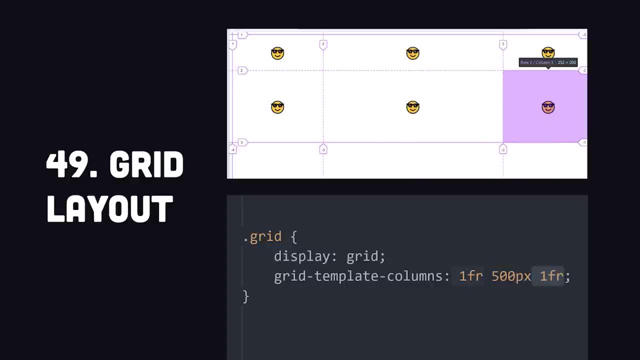 This allows search engines to display results properly and also helps with accessibility for devices like screen readers that allow anybody, regardless of disability, to enjoy the content. This allows search engines to display results properly and also helps with accessibility for devices like screen readers that allow anybody, regardless of disability, to enjoy the content. 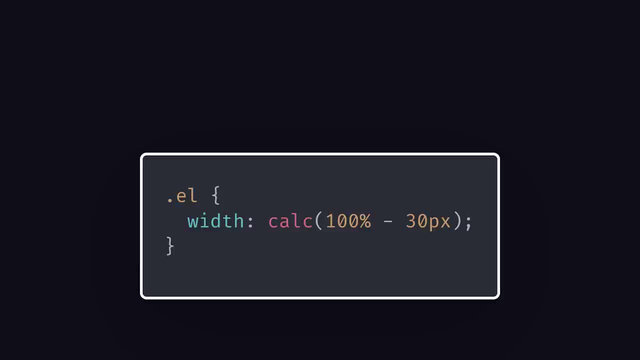 This allows search engines to display results properly and also helps with accessibility for devices like screen readers that allow anybody, regardless of disability, to enjoy the content. This allows search engines to display results properly and also helps with accessibility for devices like screen readers that allow anybody, regardless of disability, to enjoy the content. 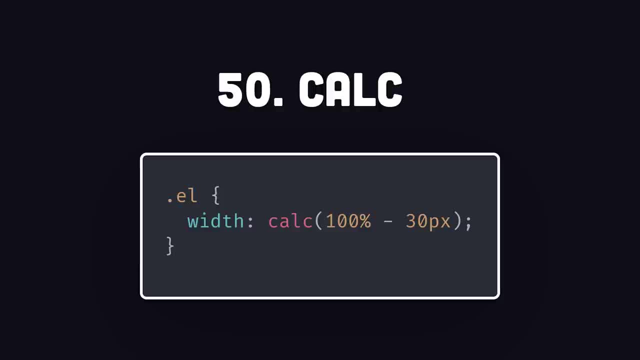 This allows search engines to display results properly and also helps with accessibility for devices like screen readers that allow anybody, regardless of disability, to enjoy the content. This allows search engines to display results properly and also helps with accessibility for devices like screen readers that allow anybody, regardless of disability, to enjoy the content. 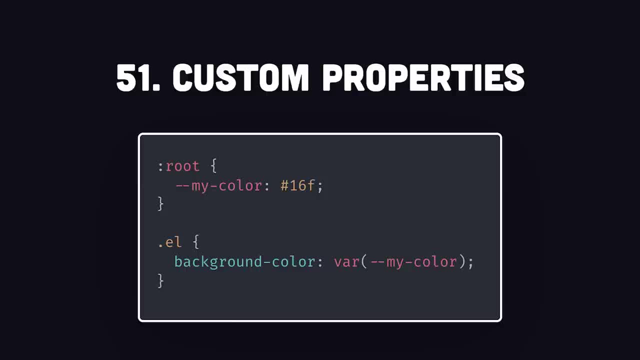 This allows search engines to display results properly and also helps with accessibility for devices like screen readers that allow anybody, regardless of disability, to enjoy the content. This allows search engines to display results properly and also helps with accessibility for devices like screen readers that allow anybody, regardless of disability, to enjoy the content. 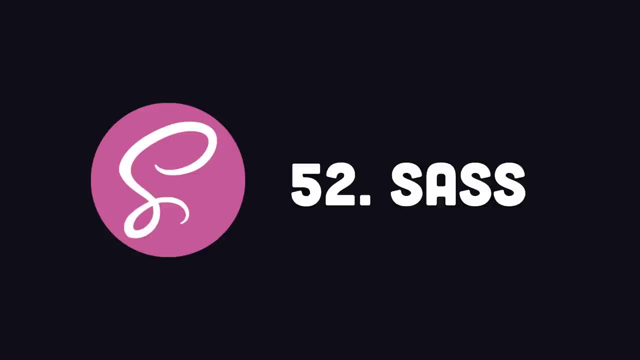 This allows search engines to display results properly and also helps with accessibility for devices like screen readers that allow anybody, regardless of disability, to enjoy the content. This allows search engines to display results properly and also helps with accessibility for devices like screen readers that allow anybody, regardless of disability, to enjoy the content. 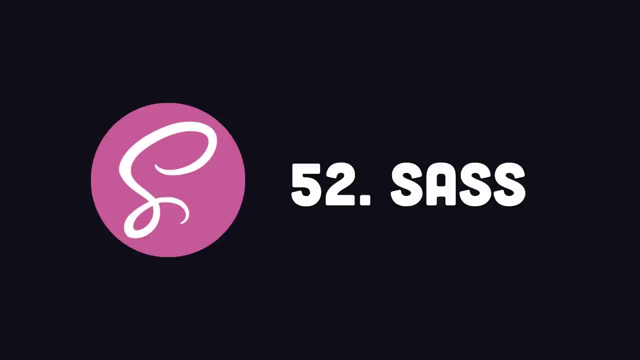 This allows search engines to display results properly and also helps with accessibility for devices like screen readers that allow anybody, regardless of disability, to enjoy the content. This allows search engines to display results properly and also helps with accessibility for devices like screen readers that allow anybody, regardless of disability, to enjoy the content. 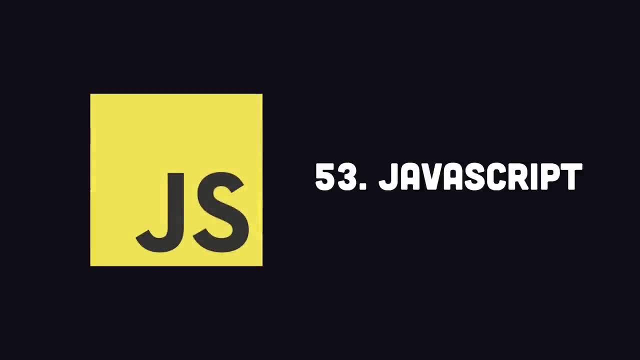 This allows search engines to display results properly and also helps with accessibility for devices like screen readers that allow anybody, regardless of disability, to enjoy the content. This allows search engines to display results properly and also helps with accessibility for devices like screen readers that allow anybody, regardless of disability, to enjoy the content. 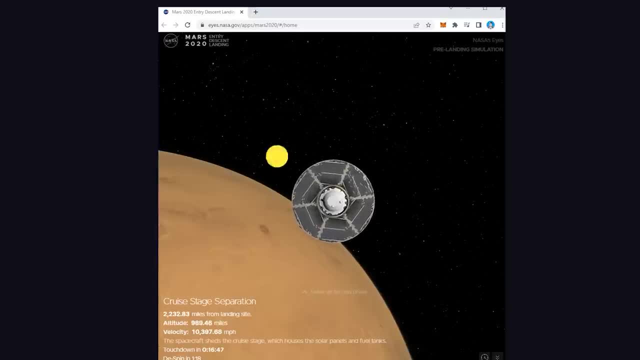 This allows search engines to display results properly and also helps with accessibility for devices like screen readers that allow anybody, regardless of disability, to enjoy the content. This allows search engines to display results properly and also helps with accessibility for devices like screen readers that allow anybody, regardless of disability, to enjoy the content. 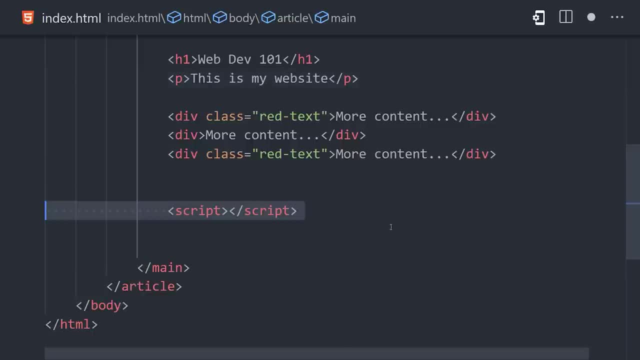 This allows search engines to display results properly and also helps with accessibility for devices like screen readers that allow anybody, regardless of disability, to enjoy the content. This allows search engines to display results properly and also helps with accessibility for devices like screen readers that allow anybody, regardless of disability, to enjoy the content. 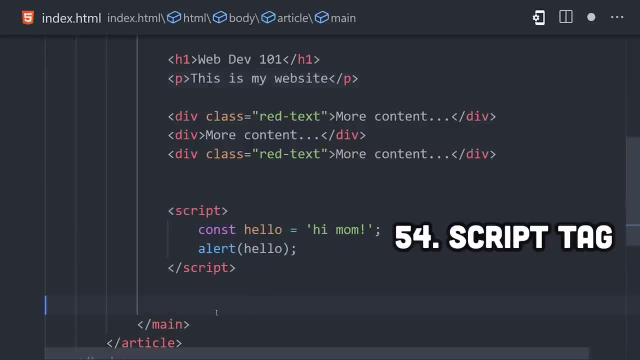 This allows search engines to display results properly and also helps with accessibility for devices like screen readers that allow anybody, regardless of disability, to enjoy the content. This allows search engines to display results properly and also helps with accessibility for devices like screen readers that allow anybody, regardless of disability, to enjoy the content. 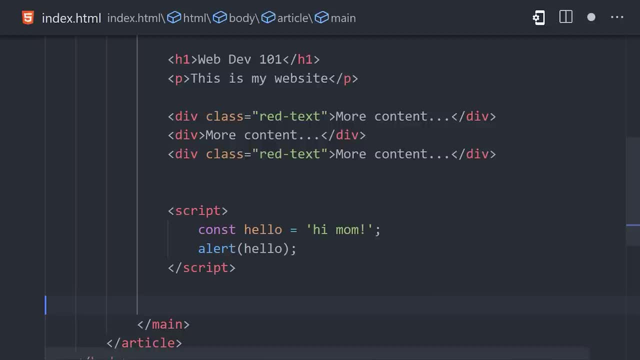 This allows search engines to display results properly and also helps with accessibility for devices like screen readers that allow anybody, regardless of disability, to enjoy the content. This allows search engines to display results properly and also helps with accessibility for devices like screen readers that allow anybody, regardless of disability, to enjoy the content. 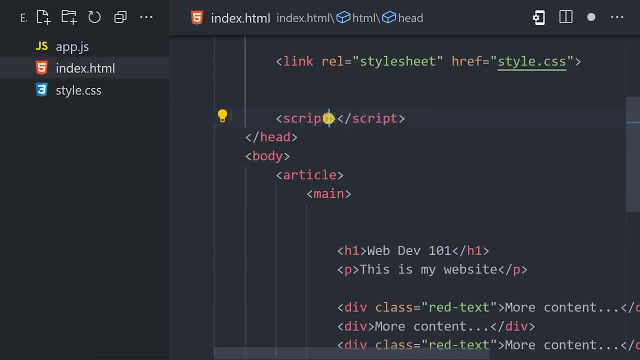 This allows search engines to display results properly and also helps with accessibility for devices like screen readers that allow anybody, regardless of disability, to enjoy the content. This allows search engines to display results properly and also helps with accessibility for devices like screen readers that allow anybody, regardless of disability, to enjoy the content. 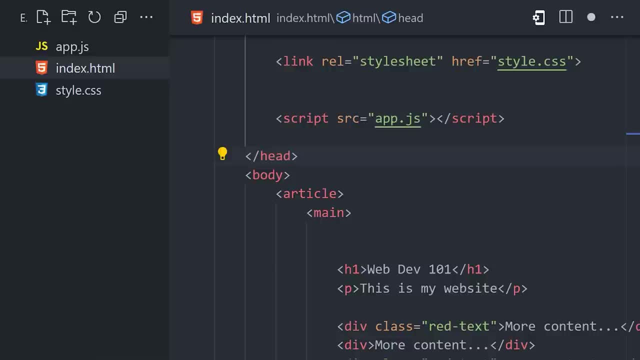 This allows search engines to display results properly and also helps with accessibility for devices like screen readers that allow anybody, regardless of disability, to enjoy the content. This allows search engines to display results properly and also helps with accessibility for devices like screen readers that allow anybody, regardless of disability, to enjoy the content. 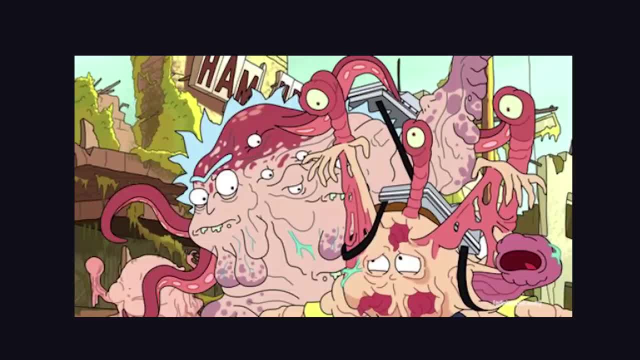 This allows search engines to display results properly and also helps with accessibility for devices like screen readers that allow anybody, regardless of disability, to enjoy the content. This allows search engines to display results properly and also helps with accessibility for devices like screen readers that allow anybody, regardless of disability, to enjoy the content. 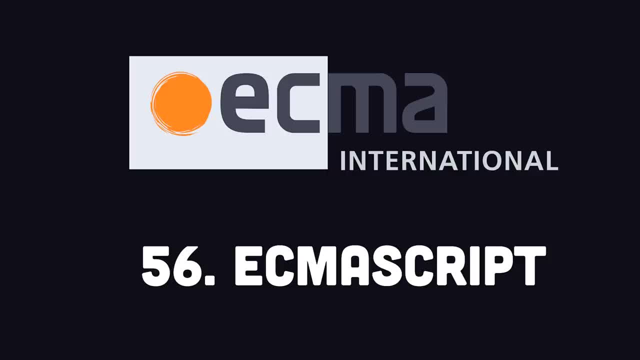 This allows search engines to display results properly and also helps with accessibility for devices like screen readers that allow anybody, regardless of disability, to enjoy the content. This allows search engines to display results properly and also helps with accessibility for devices like screen readers that allow anybody, regardless of disability, to enjoy the content. 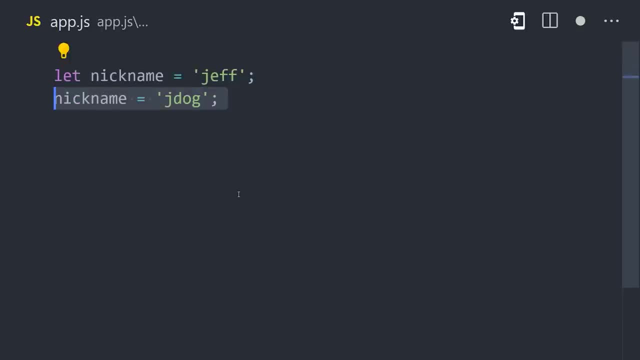 This allows search engines to display results properly and also helps with accessibility for devices like screen readers that allow anybody, regardless of disability, to enjoy the content. This allows search engines to display results properly and also helps with accessibility for devices like screen readers that allow anybody, regardless of disability, to enjoy the content. 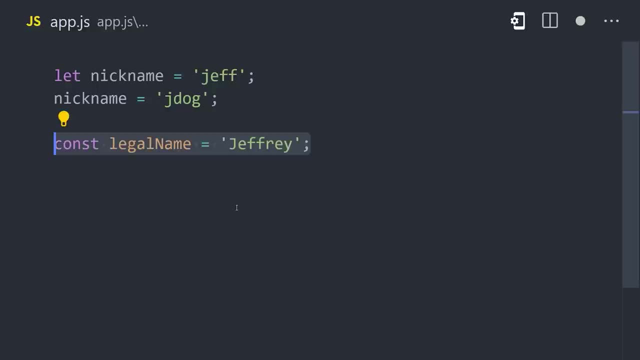 This allows search engines to display results properly and also helps with accessibility for devices like screen readers that allow anybody, regardless of disability, to enjoy the content. This allows search engines to display results properly and also helps with accessibility for devices like screen readers that allow anybody, regardless of disability, to enjoy the content. 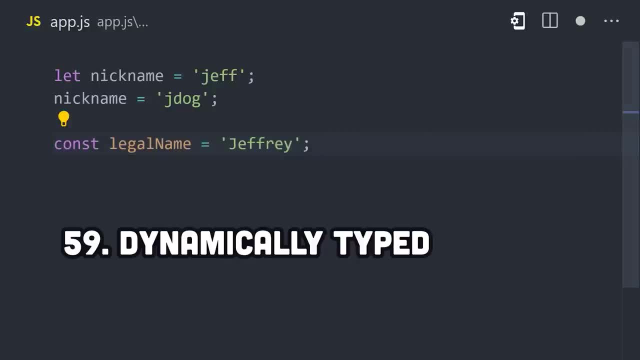 This allows search engines to display results properly and also helps with accessibility for devices like screen readers that allow anybody, regardless of disability, to enjoy the content. This allows search engines to display results properly and also helps with accessibility for devices like screen readers that allow anybody, regardless of disability, to enjoy the content. 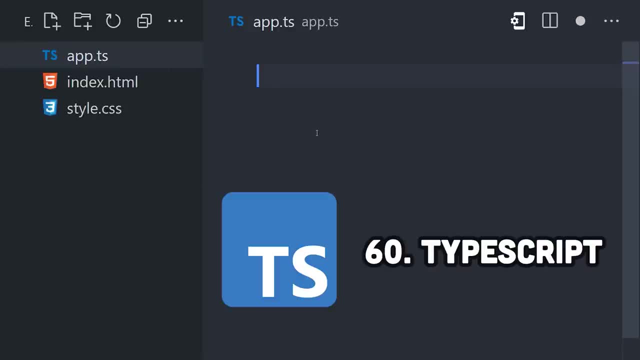 This allows search engines to display results properly and also helps with accessibility for devices like screen readers that allow anybody, regardless of disability, to enjoy the content. This allows search engines to display results properly and also helps with accessibility for devices like screen readers that allow anybody, regardless of disability, to enjoy the content. 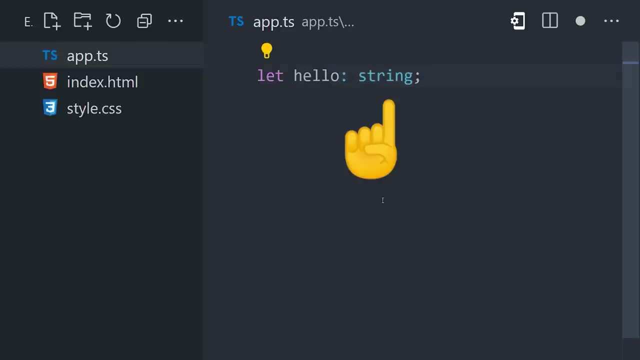 This allows search engines to display results properly and also helps with accessibility for devices like screen readers that allow anybody, regardless of disability, to enjoy the content. This allows search engines to display results properly and also helps with accessibility for devices like screen readers that allow anybody, regardless of disability, to enjoy the content. 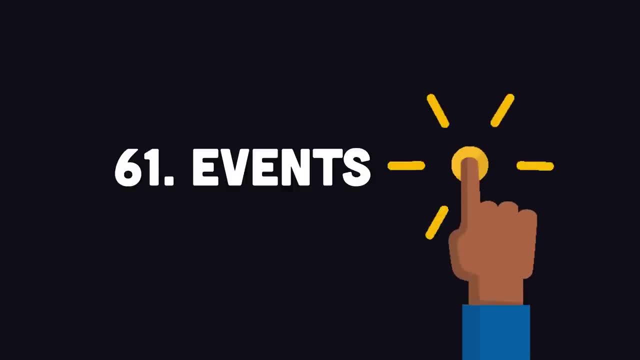 This allows search engines to display results properly and also helps with accessibility for devices like screen readers that allow anybody, regardless of disability, to enjoy the content. This allows search engines to display results properly and also helps with accessibility for devices like screen readers that allow anybody, regardless of disability, to enjoy the content. 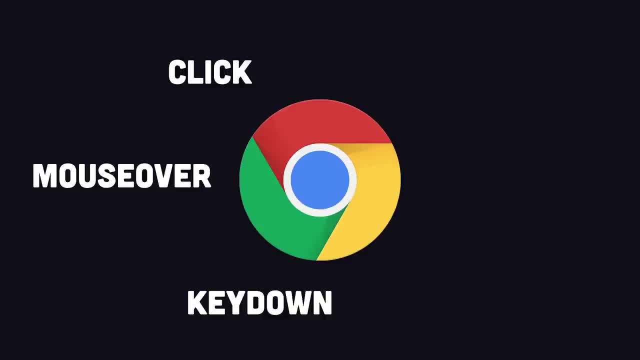 This allows search engines to display results properly and also helps with accessibility for devices like screen readers that allow anybody, regardless of disability, to enjoy the content. This allows search engines to display results properly and also helps with accessibility for devices like screen readers that allow anybody, regardless of disability, to enjoy the content. 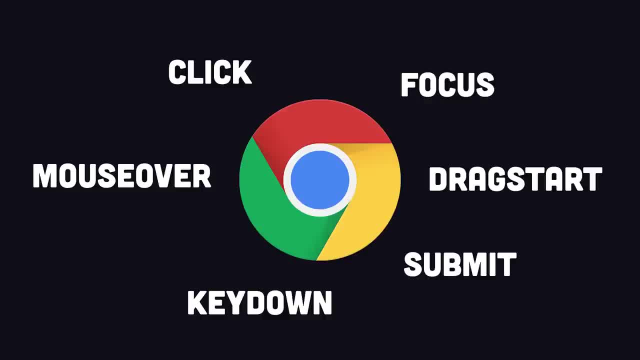 This allows search engines to display results properly and also helps with accessibility for devices like screen readers that allow anybody, regardless of disability, to enjoy the content. This allows search engines to display results properly and also helps with accessibility for devices like screen readers that allow anybody, regardless of disability, to enjoy the content. 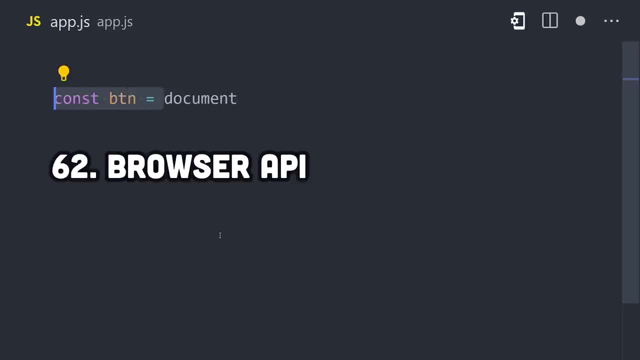 This allows search engines to display results properly and also helps with accessibility for devices like screen readers that allow anybody, regardless of disability, to enjoy the content. This allows search engines to display results properly and also helps with accessibility for devices like screen readers that allow anybody, regardless of disability, to enjoy the content. 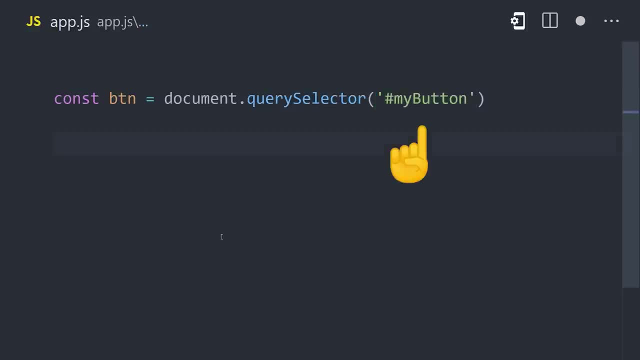 This allows search engines to display results properly and also helps with accessibility for devices like screen readers that allow anybody, regardless of disability, to enjoy the content. This allows search engines to display results properly and also helps with accessibility for devices like screen readers that allow anybody, regardless of disability, to enjoy the content. 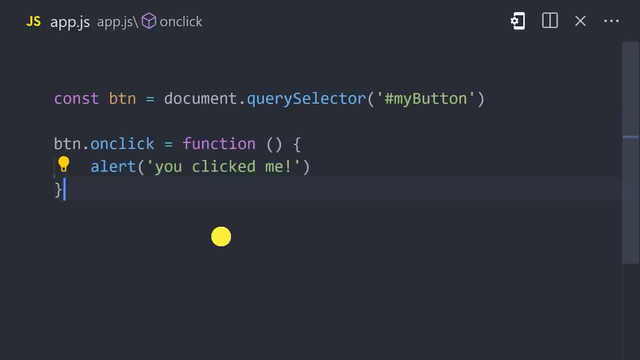 This allows search engines to display results properly and also helps with accessibility for devices like screen readers that allow anybody, regardless of disability, to enjoy the content. This allows search engines to display results properly and also helps with accessibility for devices like screen readers that allow anybody, regardless of disability, to enjoy the content. 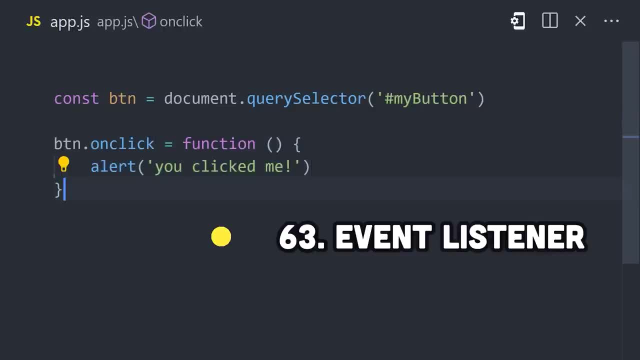 This allows search engines to display results properly and also helps with accessibility for devices like screen readers that allow anybody, regardless of disability, to enjoy the content. This allows search engines to display results properly and also helps with accessibility for devices like screen readers that allow anybody, regardless of disability, to enjoy the content. 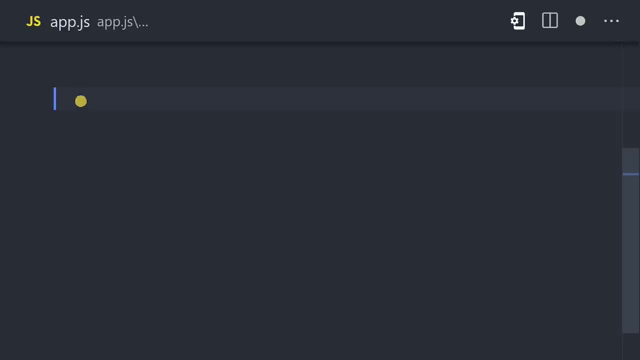 This allows search engines to display results properly and also helps with accessibility for devices like screen readers that allow anybody, regardless of disability, to enjoy the content. This allows search engines to display results properly and also helps with accessibility for devices like screen readers that allow anybody, regardless of disability, to enjoy the content. 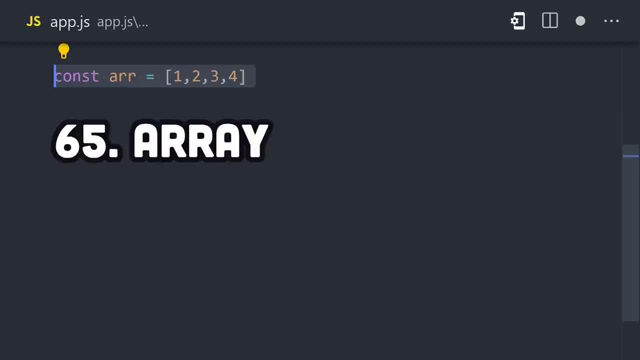 This allows search engines to display results properly and also helps with accessibility for devices like screen readers that allow anybody, regardless of disability, to enjoy the content. This allows search engines to display results properly and also helps with accessibility for devices like screen readers that allow anybody, regardless of disability, to enjoy the content. 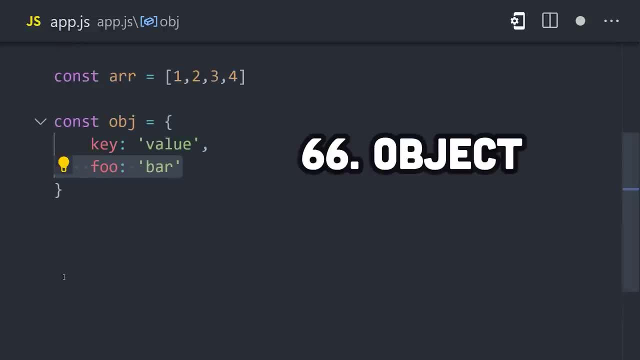 This allows search engines to display results properly and also helps with accessibility for devices like screen readers that allow anybody, regardless of disability, to enjoy the content. This allows search engines to display results properly and also helps with accessibility for devices like screen readers that allow anybody, regardless of disability, to enjoy the content. 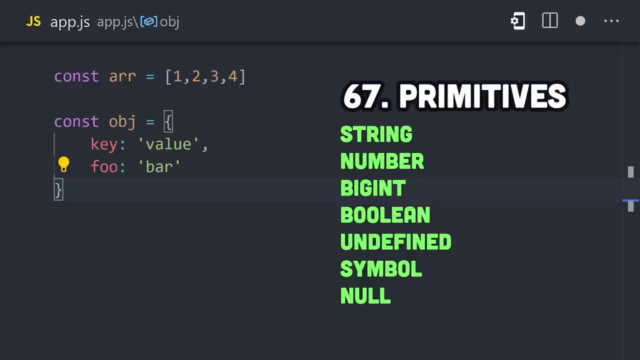 This allows search engines to display results properly and also helps with accessibility for devices like screen readers that allow anybody, regardless of disability, to enjoy the content. This allows search engines to display results properly and also helps with accessibility for devices like screen readers that allow anybody, regardless of disability, to enjoy the content. 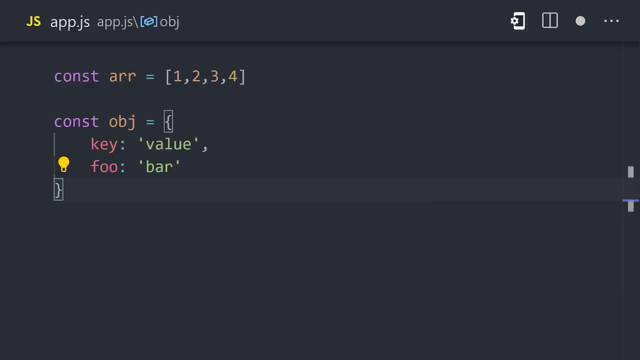 This allows search engines to display results properly and also helps with accessibility for devices like screen readers that allow anybody, regardless of disability, to enjoy the content. This allows search engines to display results properly and also helps with accessibility for devices like screen readers that allow anybody, regardless of disability, to enjoy the content. 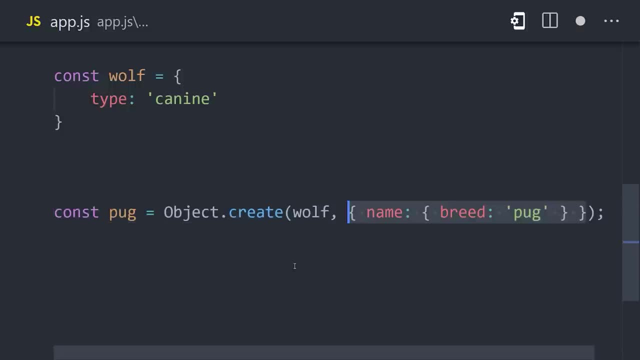 This allows search engines to display results properly and also helps with accessibility for devices like screen readers that allow anybody, regardless of disability, to enjoy the content. This allows search engines to display results properly and also helps with accessibility for devices like screen readers that allow anybody, regardless of disability, to enjoy the content. 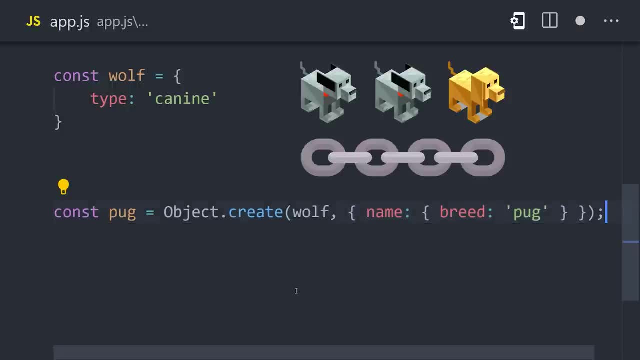 This allows search engines to display results properly and also helps with accessibility for devices like screen readers that allow anybody, regardless of disability, to enjoy the content. This allows search engines to display results properly and also helps with accessibility for devices like screen readers that allow anybody, regardless of disability, to enjoy the content. 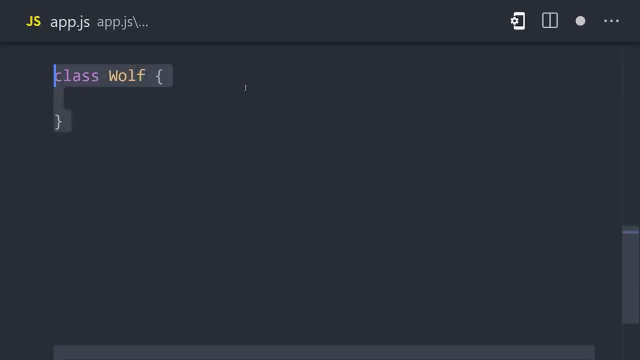 This allows search engines to display results properly and also helps with accessibility for devices like screen readers that allow anybody, regardless of disability, to enjoy the content. This allows search engines to display results properly and also helps with accessibility for devices like screen readers that allow anybody, regardless of disability, to enjoy the content. 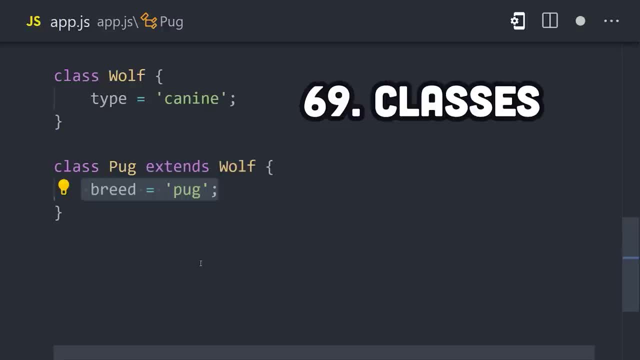 This allows search engines to display results properly and also helps with accessibility for devices like screen readers that allow anybody, regardless of disability, to enjoy the content. This allows search engines to display results properly and also helps with accessibility for devices like screen readers that allow anybody, regardless of disability, to enjoy the content. 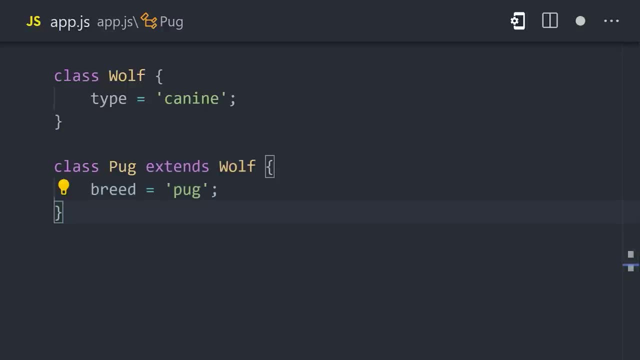 This allows search engines to display results properly and also helps with accessibility for devices like screen readers that allow anybody, regardless of disability, to enjoy the content. This allows search engines to display results properly and also helps with accessibility for devices like screen readers that allow anybody, regardless of disability, to enjoy the content. 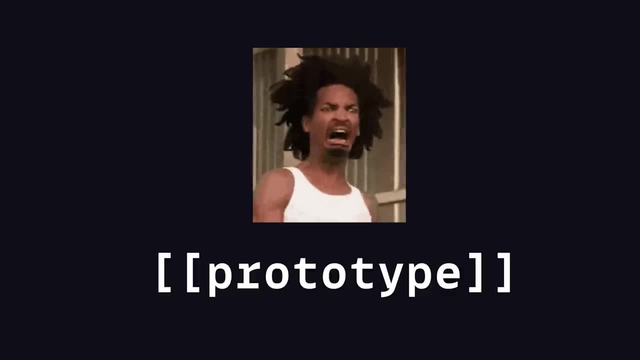 This allows search engines to display results properly and also helps with accessibility for devices like screen readers that allow anybody, regardless of disability, to enjoy the content. This allows search engines to display results properly and also helps with accessibility for devices like screen readers that allow anybody, regardless of disability, to enjoy the content. 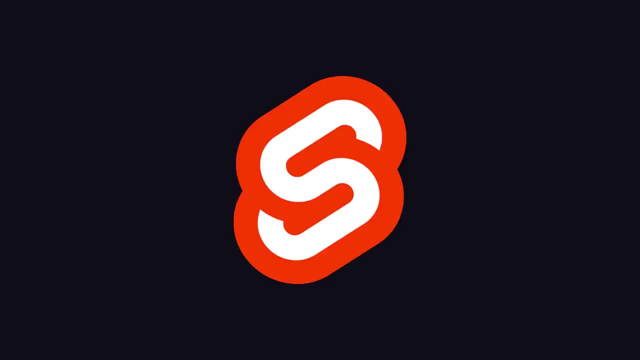 This allows search engines to display results properly and also helps with accessibility for devices like screen readers that allow anybody, regardless of disability, to enjoy the content. This allows search engines to display results properly and also helps with accessibility for devices like screen readers that allow anybody, regardless of disability, to enjoy the content. 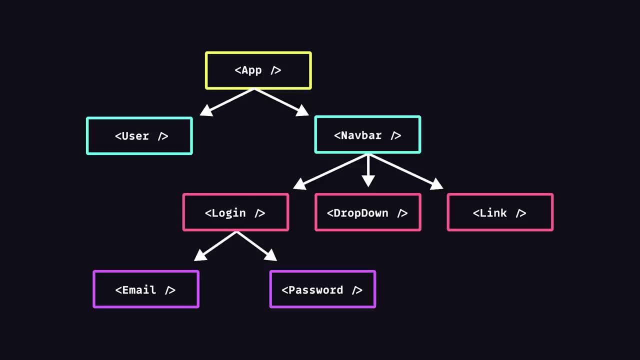 This allows search engines to display results properly and also helps with accessibility for devices like screen readers that allow anybody, regardless of disability, to enjoy the content. This allows search engines to display results properly and also helps with accessibility for devices like screen readers that allow anybody, regardless of disability, to enjoy the content. 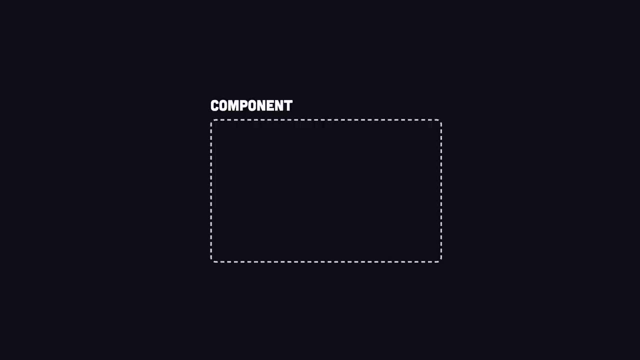 This allows search engines to display results properly and also helps with accessibility for devices like screen readers that allow anybody, regardless of disability, to enjoy the content. This allows search engines to display results properly and also helps with accessibility for devices like screen readers that allow anybody, regardless of disability, to enjoy the content. 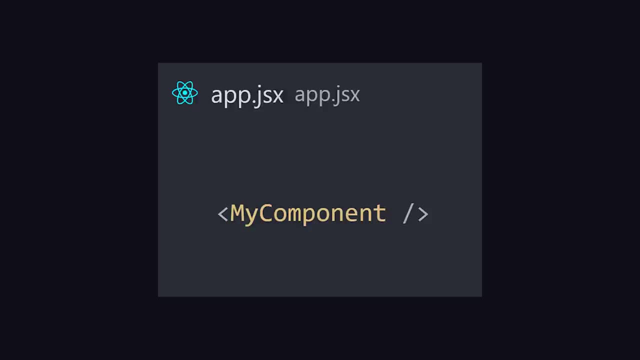 This allows search engines to display results properly and also helps with accessibility for devices like screen readers that allow anybody, regardless of disability, to enjoy the content. This allows search engines to display results properly and also helps with accessibility for devices like screen readers that allow anybody, regardless of disability, to enjoy the content. 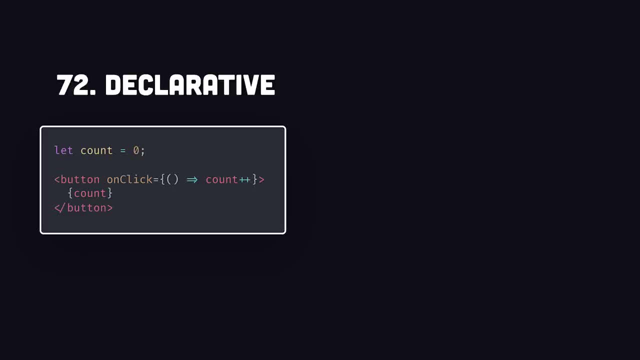 This allows search engines to display results properly and also helps with accessibility for devices like screen readers that allow anybody, regardless of disability, to enjoy the content. This allows search engines to display results properly and also helps with accessibility for devices like screen readers that allow anybody, regardless of disability, to enjoy the content. 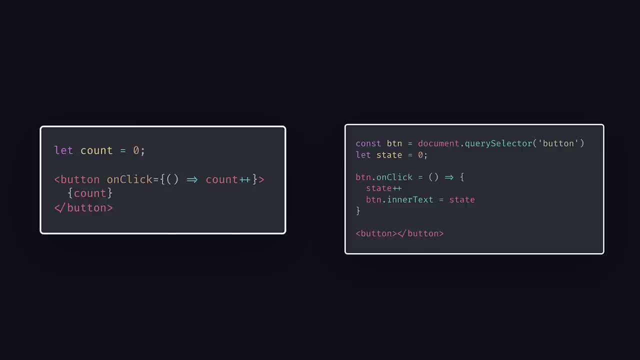 This allows search engines to display results properly and also helps with accessibility for devices like screen readers that allow anybody, regardless of disability, to enjoy the content. This allows search engines to display results properly and also helps with accessibility for devices like screen readers that allow anybody, regardless of disability, to enjoy the content. 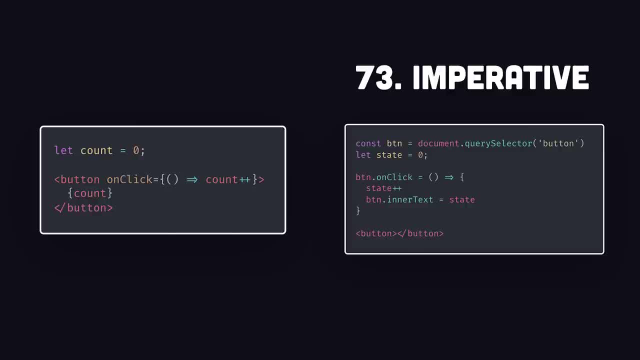 This allows search engines to display results properly and also helps with accessibility for devices like screen readers that allow anybody, regardless of disability, to enjoy the content. This allows search engines to display results properly and also helps with accessibility for devices like screen readers that allow anybody, regardless of disability, to enjoy the content. 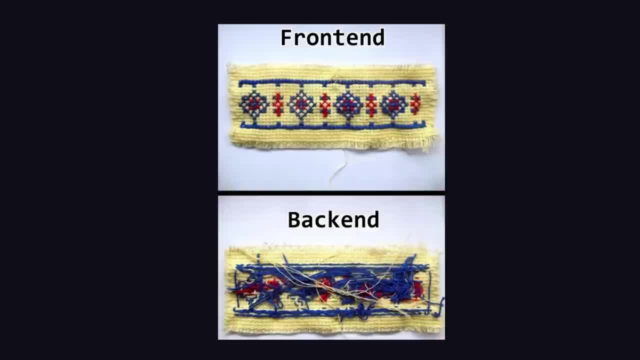 This allows search engines to display results properly and also helps with accessibility for devices like screen readers that allow anybody, regardless of disability, to enjoy the content. This allows search engines to display results properly and also helps with accessibility for devices like screen readers that allow anybody, regardless of disability, to enjoy the content. 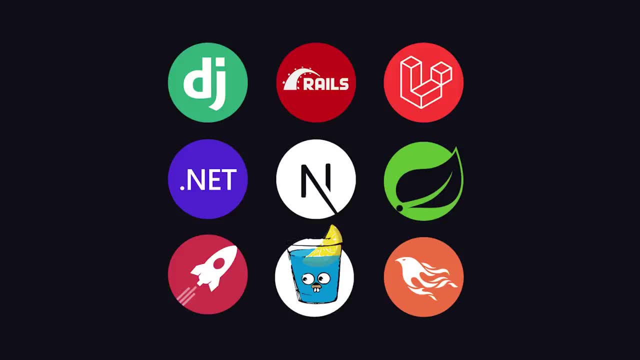 This allows search engines to display results properly and also helps with accessibility for devices like screen readers that allow anybody, regardless of disability, to enjoy the content. This allows search engines to display results properly and also helps with accessibility for devices like screen readers that allow anybody, regardless of disability, to enjoy the content. 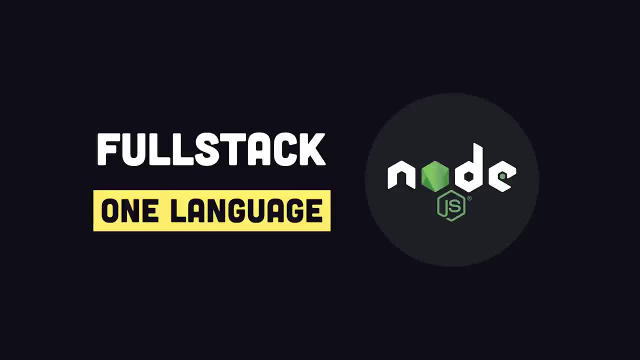 This allows search engines to display results properly and also helps with accessibility for devices like screen readers that allow anybody, regardless of disability, to enjoy the content. This allows search engines to display results properly and also helps with accessibility for devices like screen readers that allow anybody, regardless of disability, to enjoy the content. 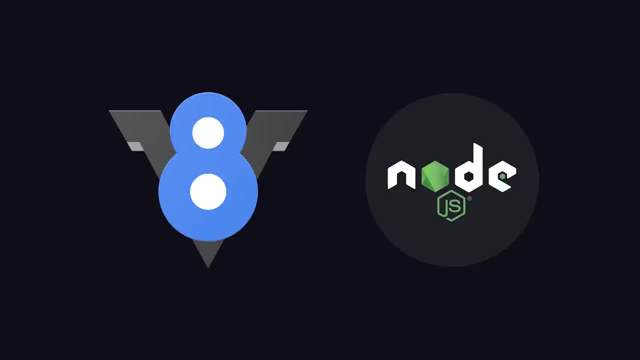 This allows search engines to display results properly and also helps with accessibility for devices like screen readers that allow anybody, regardless of disability, to enjoy the content. This allows search engines to display results properly and also helps with accessibility for devices like screen readers that allow anybody, regardless of disability, to enjoy the content. 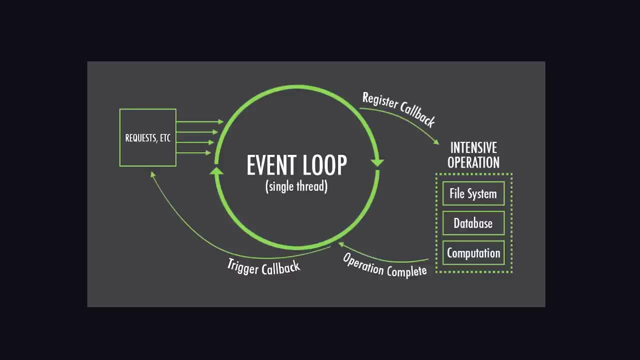 This allows search engines to display results properly and also helps with accessibility for devices like screen readers that allow anybody, regardless of disability, to enjoy the content. This allows search engines to display results properly and also helps with accessibility for devices like screen readers that allow anybody, regardless of disability, to enjoy the content. 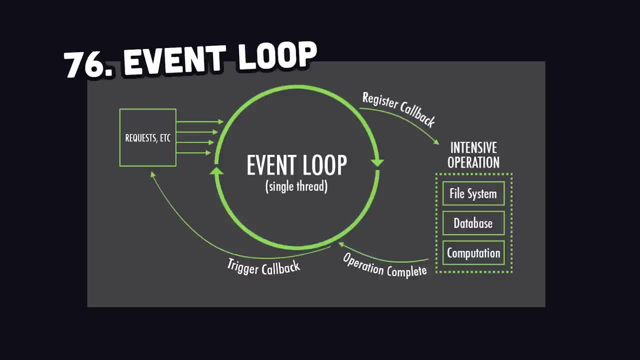 This allows search engines to display results properly and also helps with accessibility for devices like screen readers that allow anybody, regardless of disability, to enjoy the content. This allows search engines to display results properly and also helps with accessibility for devices like screen readers that allow anybody, regardless of disability, to enjoy the content. 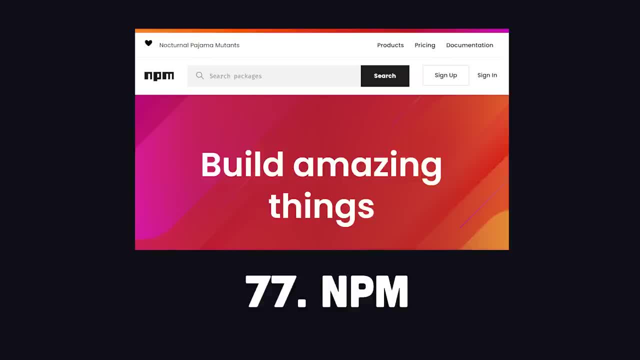 This allows search engines to display results properly and also helps with accessibility for devices like screen readers that allow anybody, regardless of disability, to enjoy the content. This allows search engines to display results properly and also helps with accessibility for devices like screen readers that allow anybody, regardless of disability, to enjoy the content. 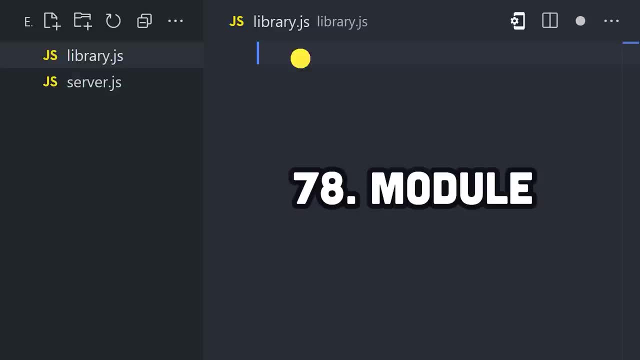 This allows search engines to display results properly and also helps with accessibility for devices like screen readers that allow anybody, regardless of disability, to enjoy the content. This allows search engines to display results properly and also helps with accessibility for devices like screen readers that allow anybody, regardless of disability, to enjoy the content. 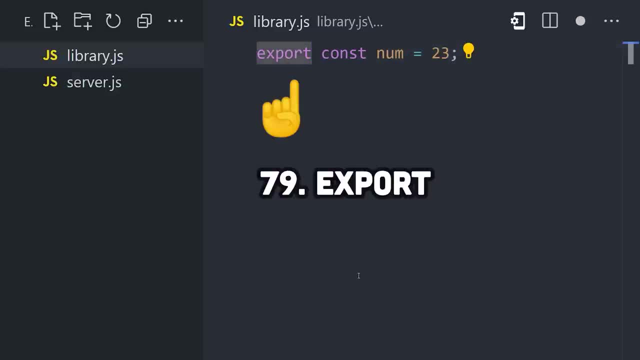 This allows search engines to display results properly and also helps with accessibility for devices like screen readers that allow anybody, regardless of disability, to enjoy the content. This allows search engines to display results properly and also helps with accessibility for devices like screen readers that allow anybody, regardless of disability, to enjoy the content. 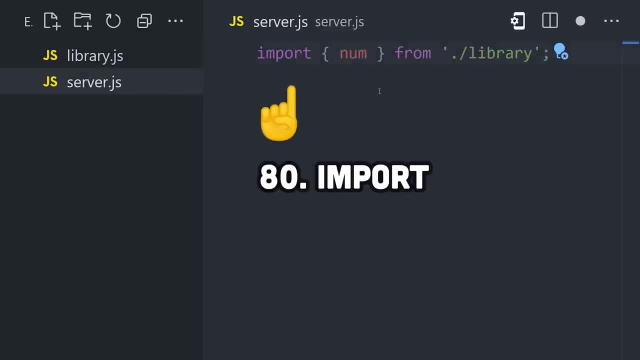 This allows search engines to display results properly and also helps with accessibility for devices like screen readers that allow anybody, regardless of disability, to enjoy the content. This allows search engines to display results properly and also helps with accessibility for devices like screen readers that allow anybody, regardless of disability, to enjoy the content. 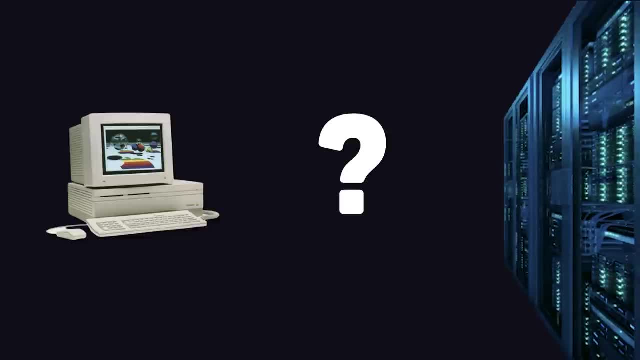 This allows search engines to display results properly and also helps with accessibility for devices like screen readers that allow anybody, regardless of disability, to enjoy the content. This allows search engines to display results properly and also helps with accessibility for devices like screen readers that allow anybody, regardless of disability, to enjoy the content. 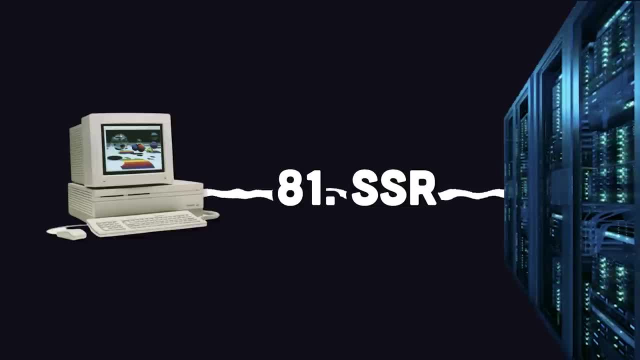 This allows search engines to display results properly and also helps with accessibility for devices like screen readers that allow anybody, regardless of disability, to enjoy the content. This allows search engines to display results properly and also helps with accessibility for devices like screen readers that allow anybody, regardless of disability, to enjoy the content. 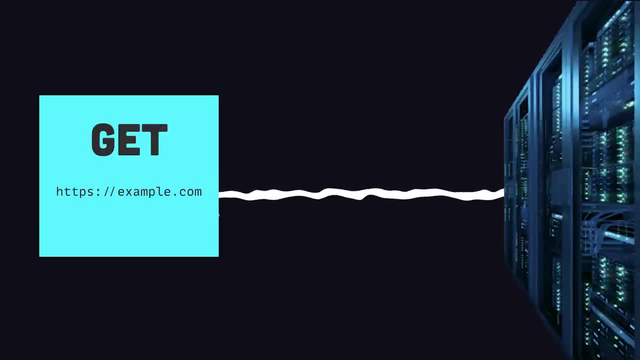 This allows search engines to display results properly and also helps with accessibility for devices like screen readers that allow anybody, regardless of disability, to enjoy the content. This allows search engines to display results properly and also helps with accessibility for devices like screen readers that allow anybody, regardless of disability, to enjoy the content. 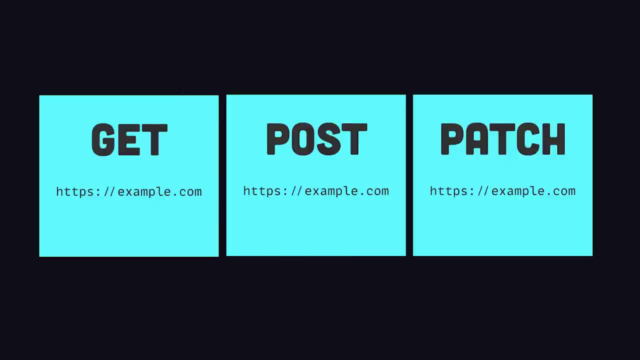 This allows search engines to display results properly and also helps with accessibility for devices like screen readers that allow anybody, regardless of disability, to enjoy the content. This allows search engines to display results properly and also helps with accessibility for devices like screen readers that allow anybody, regardless of disability, to enjoy the content. 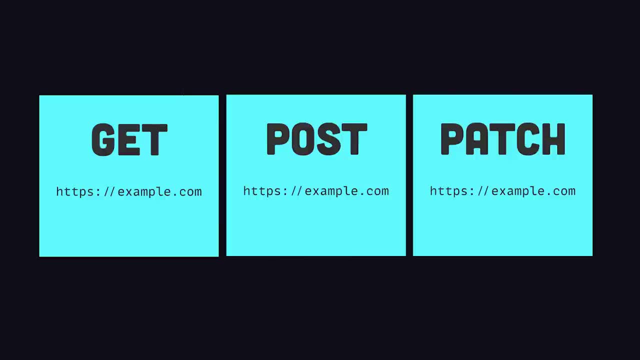 This allows search engines to display results properly and also helps with accessibility for devices like screen readers that allow anybody, regardless of disability, to enjoy the content. This allows search engines to display results properly and also helps with accessibility for devices like screen readers that allow anybody, regardless of disability, to enjoy the content. 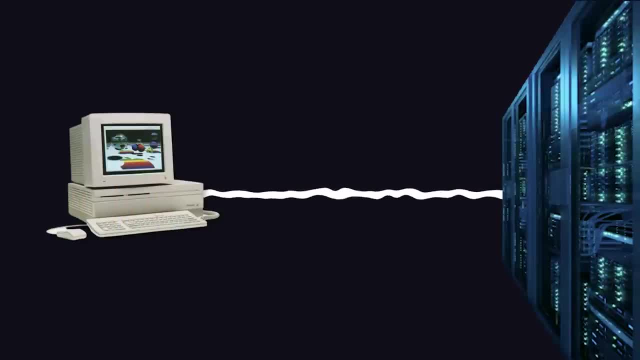 This allows search engines to display results properly and also helps with accessibility for devices like screen readers that allow anybody, regardless of disability, to enjoy the content. This allows search engines to display results properly and also helps with accessibility for devices like screen readers that allow anybody, regardless of disability, to enjoy the content. 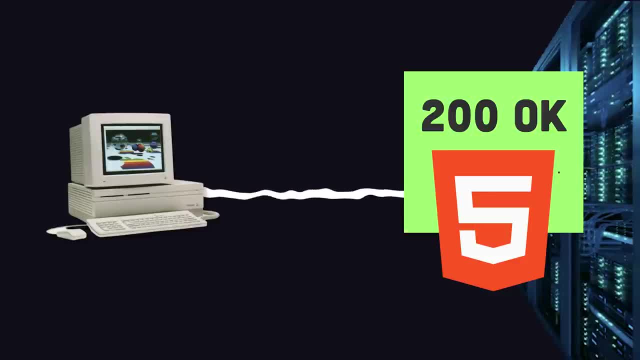 This allows search engines to display results properly and also helps with accessibility for devices like screen readers that allow anybody, regardless of disability, to enjoy the content. This allows search engines to display results properly and also helps with accessibility for devices like screen readers that allow anybody, regardless of disability, to enjoy the content. 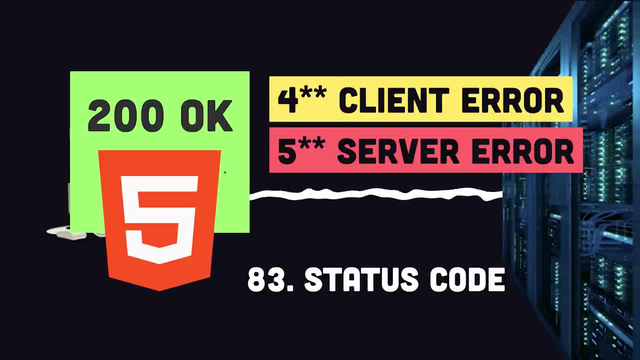 This allows search engines to display results properly and also helps with accessibility for devices like screen readers that allow anybody, regardless of disability, to enjoy the content. This allows search engines to display results properly and also helps with accessibility for devices like screen readers that allow anybody, regardless of disability, to enjoy the content. 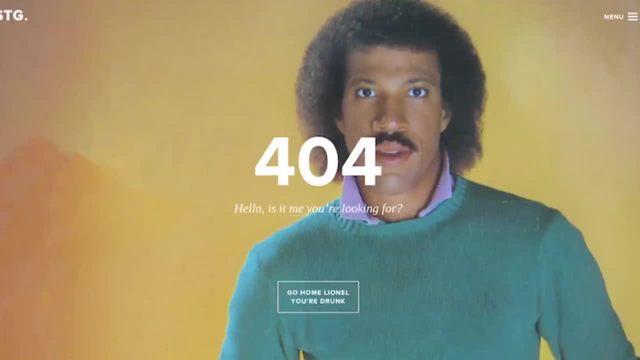 This allows search engines to display results properly and also helps with accessibility for devices like screen readers that allow anybody, regardless of disability, to enjoy the content. This allows search engines to display results properly and also helps with accessibility for devices like screen readers that allow anybody, regardless of disability, to enjoy the content. 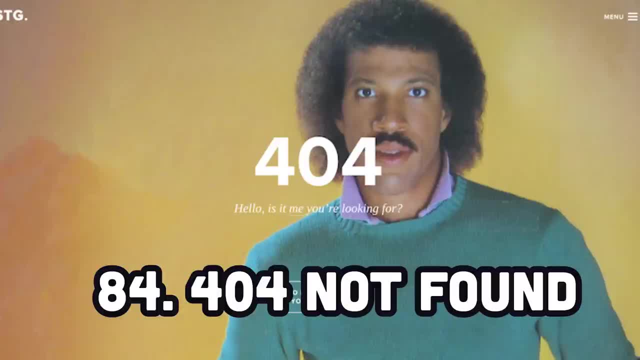 This allows search engines to display results properly and also helps with accessibility for devices like screen readers that allow anybody, regardless of disability, to enjoy the content. This allows search engines to display results properly and also helps with accessibility for devices like screen readers that allow anybody, regardless of disability, to enjoy the content. 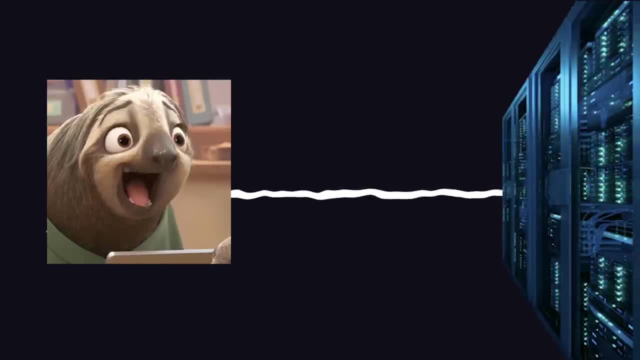 This allows search engines to display results properly and also helps with accessibility for devices like screen readers that allow anybody, regardless of disability, to enjoy the content. This allows search engines to display results properly and also helps with accessibility for devices like screen readers that allow anybody, regardless of disability, to enjoy the content. 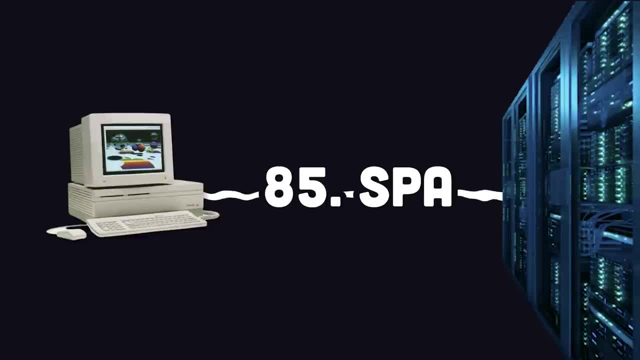 This allows search engines to display results properly and also helps with accessibility for devices like screen readers that allow anybody, regardless of disability, to enjoy the content. This allows search engines to display results properly and also helps with accessibility for devices like screen readers that allow anybody, regardless of disability, to enjoy the content. 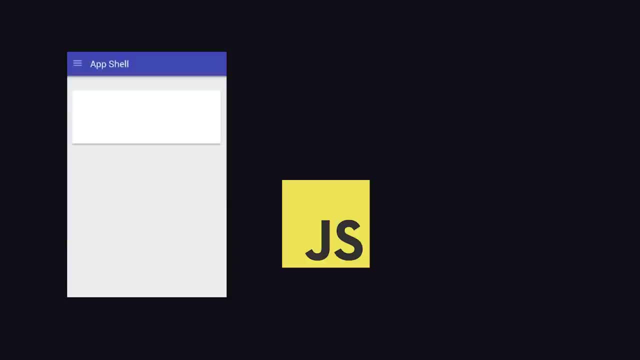 This allows search engines to display results properly and also helps with accessibility for devices like screen readers that allow anybody, regardless of disability, to enjoy the content. This allows search engines to display results properly and also helps with accessibility for devices like screen readers that allow anybody, regardless of disability, to enjoy the content. 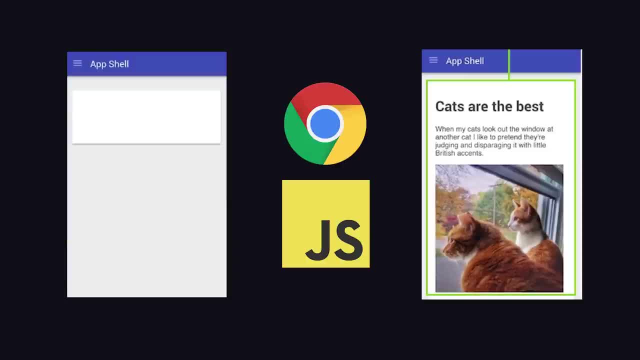 This allows search engines to display results properly and also helps with accessibility for devices like screen readers that allow anybody, regardless of disability, to enjoy the content. This allows search engines to display results properly and also helps with accessibility for devices like screen readers that allow anybody, regardless of disability, to enjoy the content. 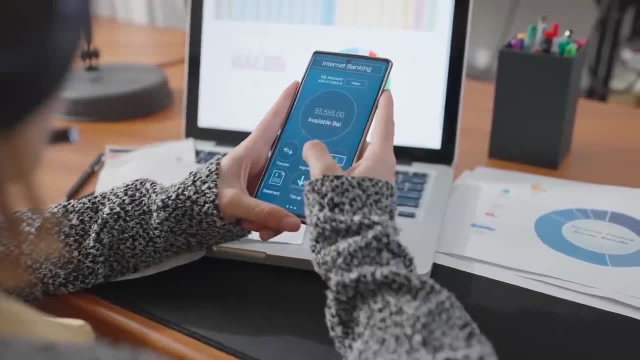 This allows search engines to display results properly and also helps with accessibility for devices like screen readers that allow anybody, regardless of disability, to enjoy the content. This allows search engines to display results properly and also helps with accessibility for devices like screen readers that allow anybody, regardless of disability, to enjoy the content. 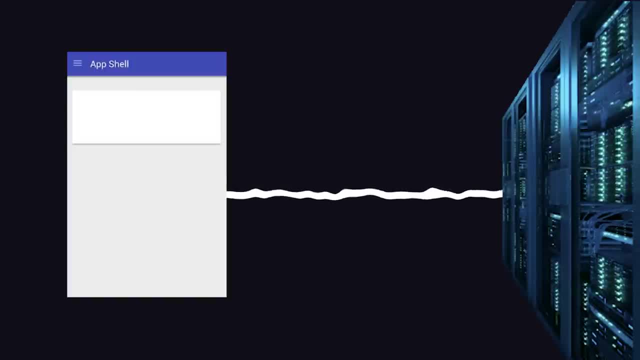 This allows search engines to display results properly and also helps with accessibility for devices like screen readers that allow anybody, regardless of disability, to enjoy the content. This allows search engines to display results properly and also helps with accessibility for devices like screen readers that allow anybody, regardless of disability, to enjoy the content. 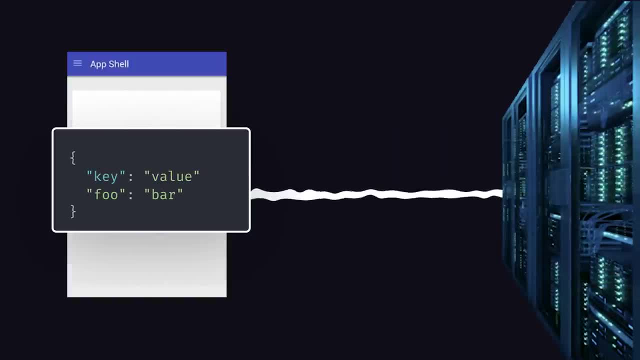 This allows search engines to display results properly and also helps with accessibility for devices like screen readers that allow anybody, regardless of disability, to enjoy the content. This allows search engines to display results properly and also helps with accessibility for devices like screen readers that allow anybody, regardless of disability, to enjoy the content. 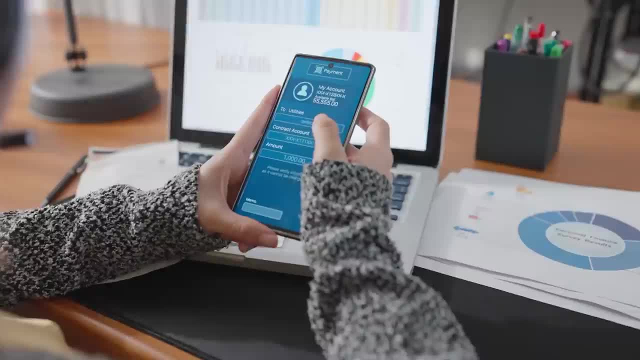 This allows search engines to display results properly and also helps with accessibility for devices like screen readers that allow anybody, regardless of disability, to enjoy the content. This allows search engines to display results properly and also helps with accessibility for devices like screen readers that allow anybody, regardless of disability, to enjoy the content. 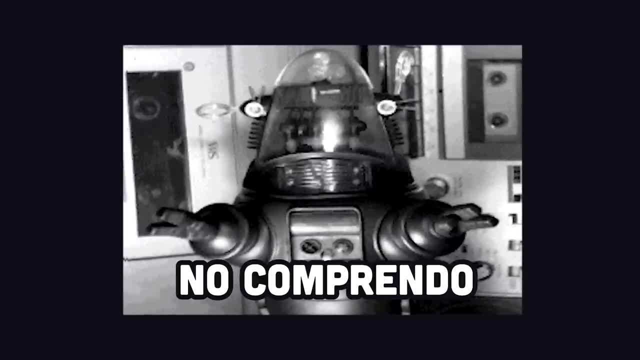 This allows search engines to display results properly and also helps with accessibility for devices like screen readers that allow anybody, regardless of disability, to enjoy the content. This allows search engines to display results properly and also helps with accessibility for devices like screen readers that allow anybody, regardless of disability, to enjoy the content. 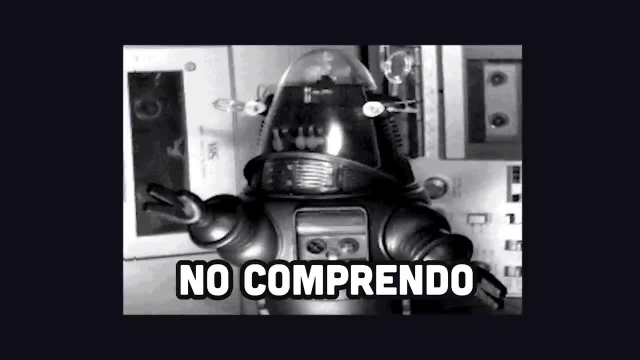 This allows search engines to display results properly and also helps with accessibility for devices like screen readers that allow anybody, regardless of disability, to enjoy the content. This allows search engines to display results properly and also helps with accessibility for devices like screen readers that allow anybody, regardless of disability, to enjoy the content. 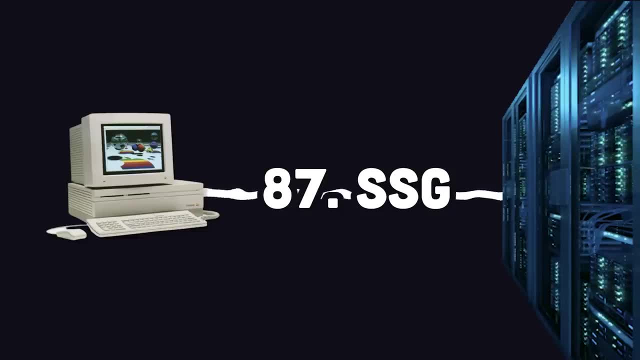 This allows search engines to display results properly and also helps with accessibility for devices like screen readers that allow anybody, regardless of disability, to enjoy the content. This allows search engines to display results properly and also helps with accessibility for devices like screen readers that allow anybody, regardless of disability, to enjoy the content. 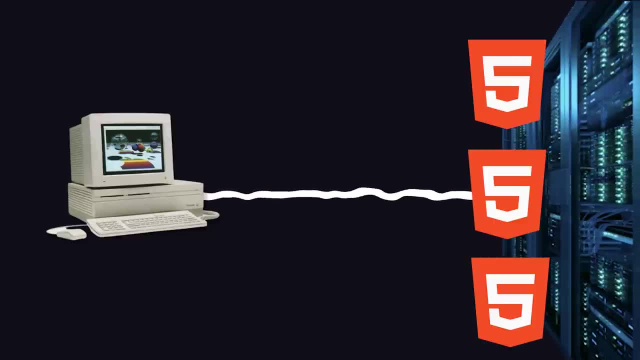 This allows search engines to display results properly and also helps with accessibility for devices like screen readers that allow anybody, regardless of disability, to enjoy the content. This allows search engines to display results properly and also helps with accessibility for devices like screen readers that allow anybody, regardless of disability, to enjoy the content. 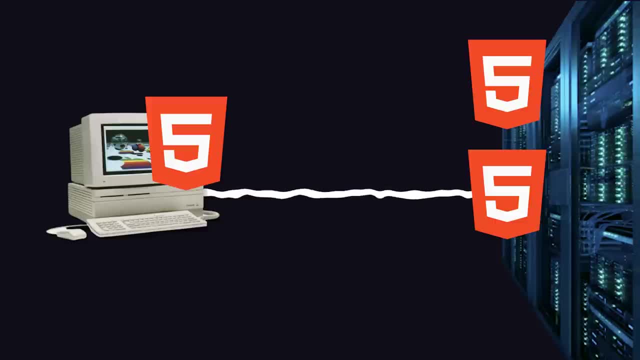 This allows search engines to display results properly and also helps with accessibility for devices like screen readers that allow anybody, regardless of disability, to enjoy the content. This allows search engines to display results properly and also helps with accessibility for devices like screen readers that allow anybody, regardless of disability, to enjoy the content. 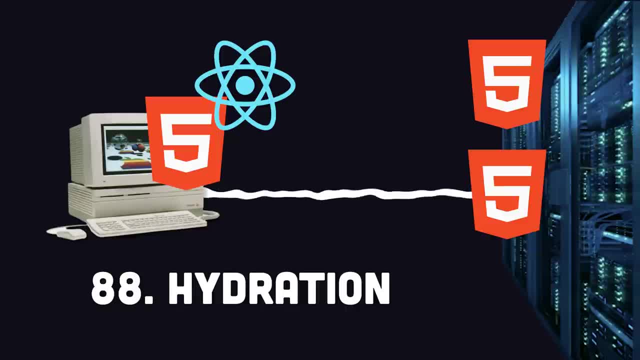 This allows search engines to display results properly and also helps with accessibility for devices like screen readers that allow anybody, regardless of disability, to enjoy the content. This allows search engines to display results properly and also helps with accessibility for devices like screen readers that allow anybody, regardless of disability, to enjoy the content. 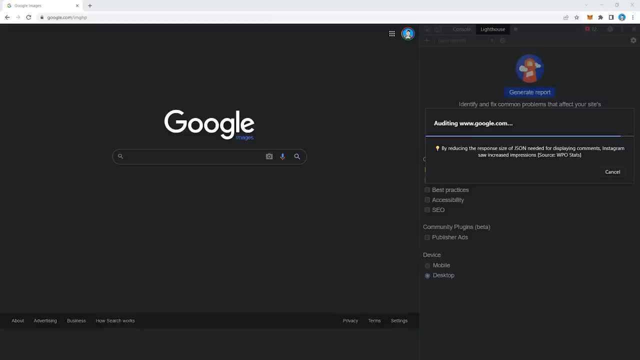 This allows search engines to display results properly and also helps with accessibility for devices like screen readers that allow anybody, regardless of disability, to enjoy the content. This allows search engines to display results properly and also helps with accessibility for devices like screen readers that allow anybody, regardless of disability, to enjoy the content. 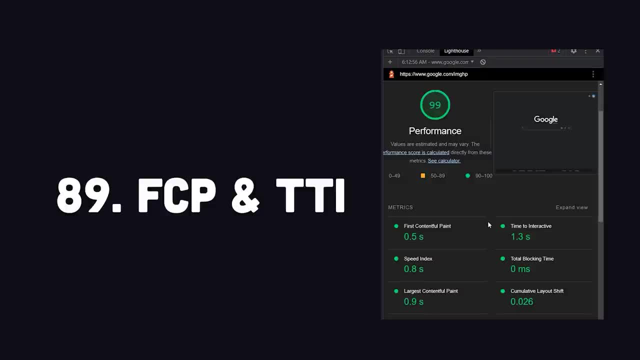 This allows search engines to display results properly and also helps with accessibility for devices like screen readers that allow anybody, regardless of disability, to enjoy the content. This allows search engines to display results properly and also helps with accessibility for devices like screen readers that allow anybody, regardless of disability, to enjoy the content. 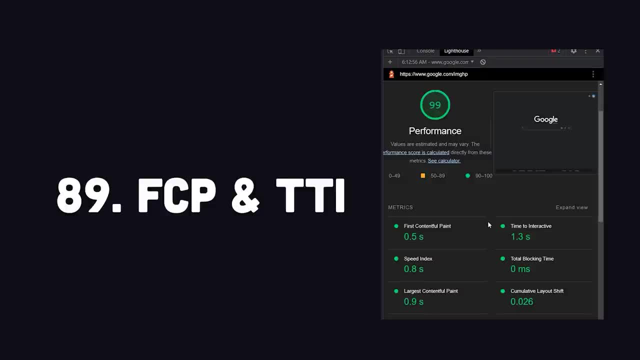 This allows search engines to display results properly and also helps with accessibility for devices like screen readers that allow anybody, regardless of disability, to enjoy the content. This allows search engines to display results properly and also helps with accessibility for devices like screen readers that allow anybody, regardless of disability, to enjoy the content. 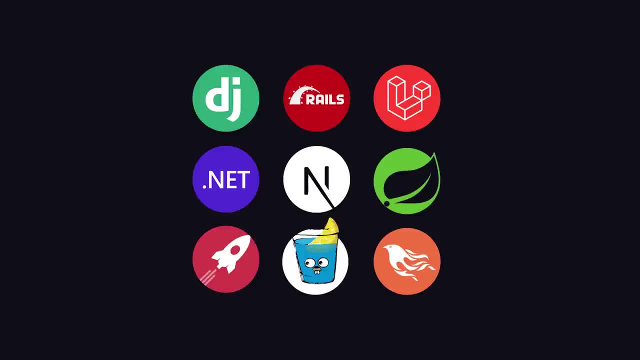 This allows search engines to display results properly and also helps with accessibility for devices like screen readers that allow anybody, regardless of disability, to enjoy the content. This allows search engines to display results properly and also helps with accessibility for devices like screen readers that allow anybody, regardless of disability, to enjoy the content. 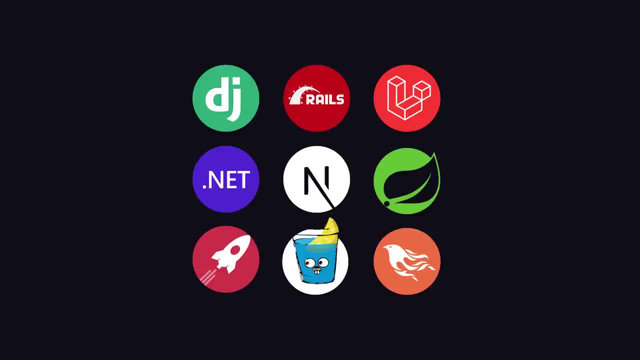 This allows search engines to display results properly and also helps with accessibility for devices like screen readers that allow anybody, regardless of disability, to enjoy the content. This allows search engines to display results properly and also helps with accessibility for devices like screen readers that allow anybody, regardless of disability, to enjoy the content. 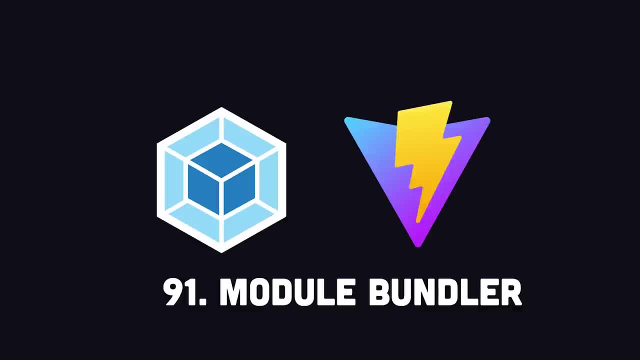 This allows search engines to display results properly and also helps with accessibility for devices like screen readers that allow anybody, regardless of disability, to enjoy the content. This allows search engines to display results properly and also helps with accessibility for devices like screen readers that allow anybody, regardless of disability, to enjoy the content. 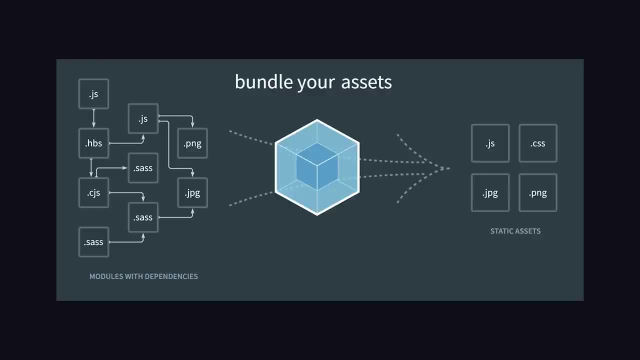 This allows search engines to display results properly and also helps with accessibility for devices like screen readers that allow anybody, regardless of disability, to enjoy the content. This allows search engines to display results properly and also helps with accessibility for devices like screen readers that allow anybody, regardless of disability, to enjoy the content. 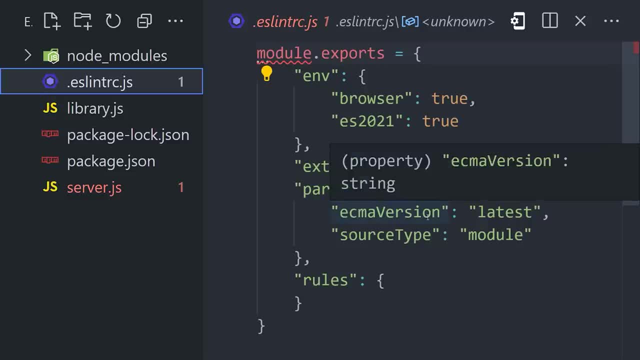 This allows search engines to display results properly and also helps with accessibility for devices like screen readers that allow anybody, regardless of disability, to enjoy the content. This allows search engines to display results properly and also helps with accessibility for devices like screen readers that allow anybody, regardless of disability, to enjoy the content. 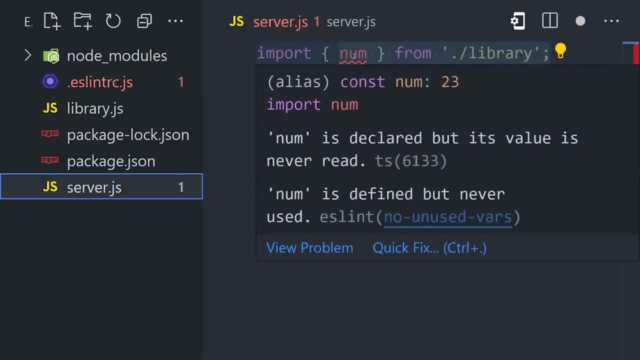 This allows search engines to display results properly and also helps with accessibility for devices like screen readers that allow anybody, regardless of disability, to enjoy the content. This allows search engines to display results properly and also helps with accessibility for devices like screen readers that allow anybody, regardless of disability, to enjoy the content. 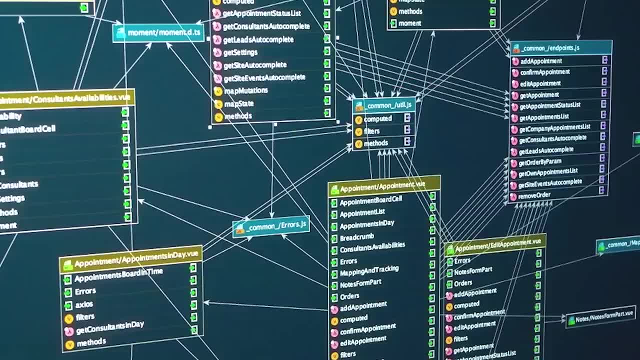 This allows search engines to display results properly and also helps with accessibility for devices like screen readers that allow anybody, regardless of disability, to enjoy the content. This allows search engines to display results properly and also helps with accessibility for devices like screen readers that allow anybody, regardless of disability, to enjoy the content. 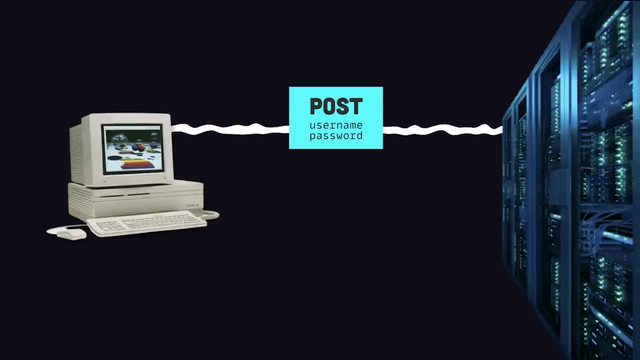 This allows search engines to display results properly and also helps with accessibility for devices like screen readers that allow anybody, regardless of disability, to enjoy the content. This allows search engines to display results properly and also helps with accessibility for devices like screen readers that allow anybody, regardless of disability, to enjoy the content. 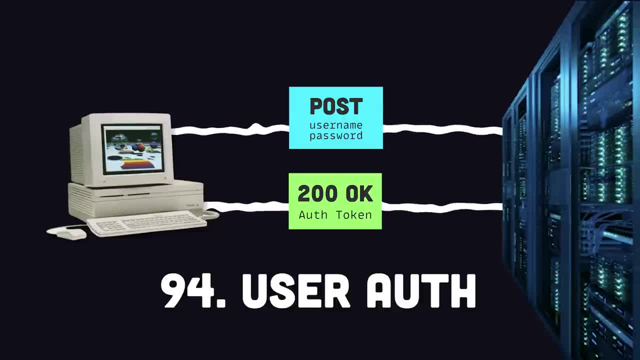 This allows search engines to display results properly and also helps with accessibility for devices like screen readers that allow anybody, regardless of disability, to enjoy the content. This allows search engines to display results properly and also helps with accessibility for devices like screen readers that allow anybody, regardless of disability, to enjoy the content. 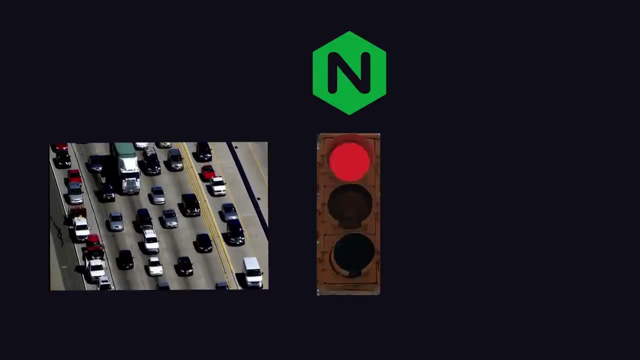 This allows search engines to display results properly and also helps with accessibility for devices like screen readers that allow anybody, regardless of disability, to enjoy the content. This allows search engines to display results properly and also helps with accessibility for devices like screen readers that allow anybody, regardless of disability, to enjoy the content. 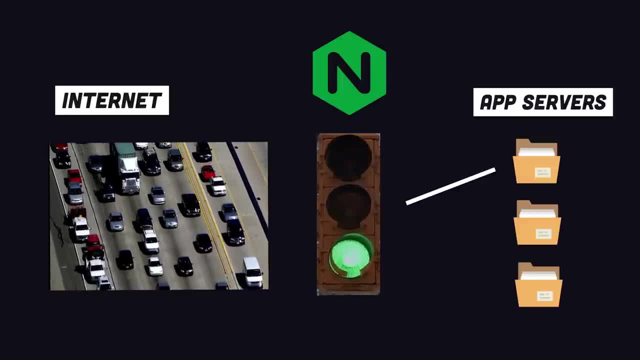 This allows search engines to display results properly and also helps with accessibility for devices like screen readers that allow anybody, regardless of disability, to enjoy the content. This allows search engines to display results properly and also helps with accessibility for devices like screen readers that allow anybody, regardless of disability, to enjoy the content. 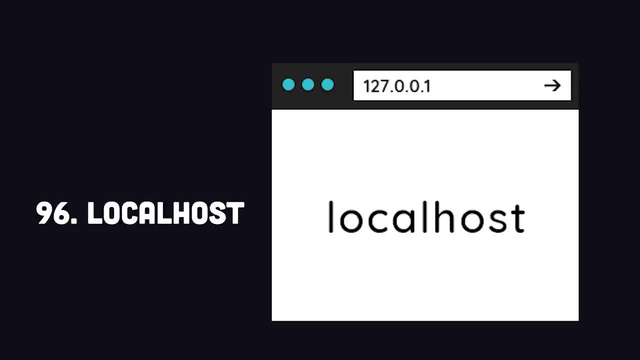 This allows search engines to display results properly and also helps with accessibility for devices like screen readers that allow anybody, regardless of disability, to enjoy the content. This allows search engines to display results properly and also helps with accessibility for devices like screen readers that allow anybody, regardless of disability, to enjoy the content. 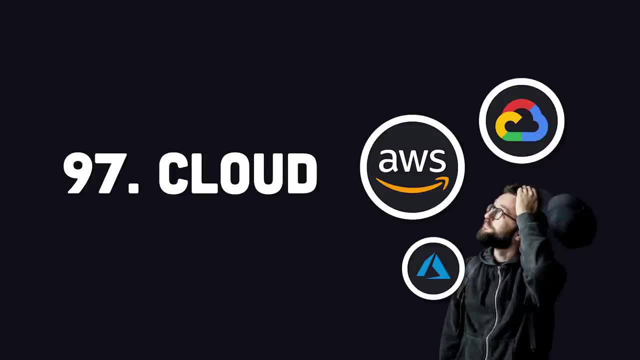 This allows search engines to display results properly and also helps with accessibility for devices like screen readers that allow anybody, regardless of disability, to enjoy the content. This allows search engines to display results properly and also helps with accessibility for devices like screen readers that allow anybody, regardless of disability, to enjoy the content. 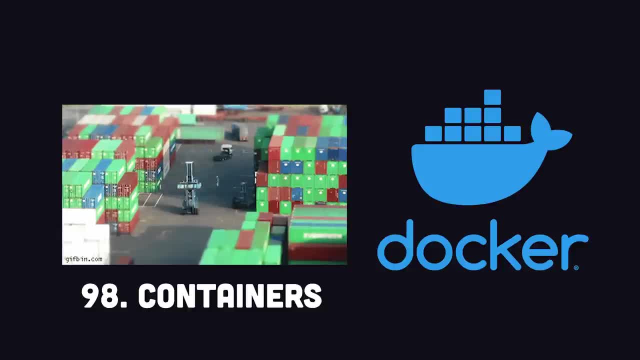 This allows search engines to display results properly and also helps with accessibility for devices like screen readers that allow anybody, regardless of disability, to enjoy the content. This allows search engines to display results properly and also helps with accessibility for devices like screen readers that allow anybody, regardless of disability, to enjoy the content. 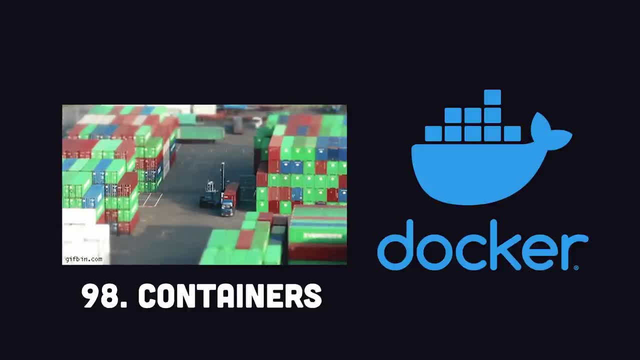 This allows search engines to display results properly and also helps with accessibility for devices like screen readers that allow anybody, regardless of disability, to enjoy the content. This allows search engines to display results properly and also helps with accessibility for devices like screen readers that allow anybody, regardless of disability, to enjoy the content. 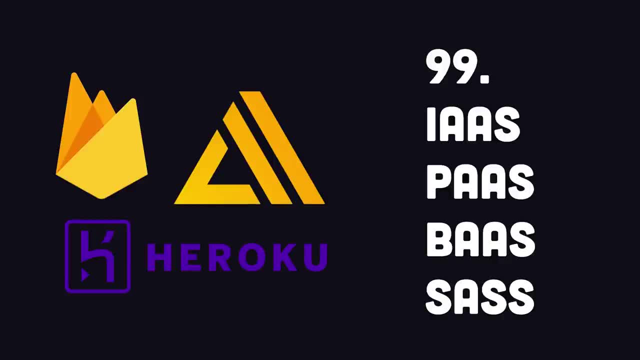 This allows search engines to display results properly and also helps with accessibility for devices like screen readers that allow anybody, regardless of disability, to enjoy the content. This allows search engines to display results properly and also helps with accessibility for devices like screen readers that allow anybody, regardless of disability, to enjoy the content. 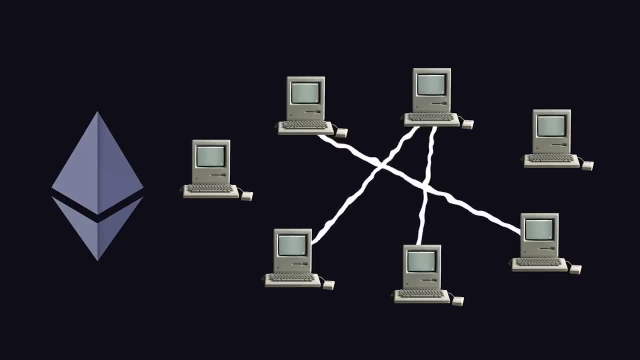 This allows search engines to display results properly and also helps with accessibility for devices like screen readers that allow anybody, regardless of disability, to enjoy the content. This allows search engines to display results properly and also helps with accessibility for devices like screen readers that allow anybody, regardless of disability, to enjoy the content. 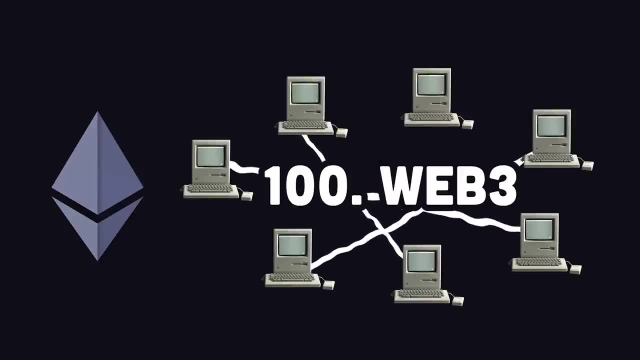 This allows search engines to display results properly and also helps with accessibility for devices like screen readers that allow anybody, regardless of disability, to enjoy the content. This allows search engines to display results properly and also helps with accessibility for devices like screen readers that allow anybody, regardless of disability, to enjoy the content. 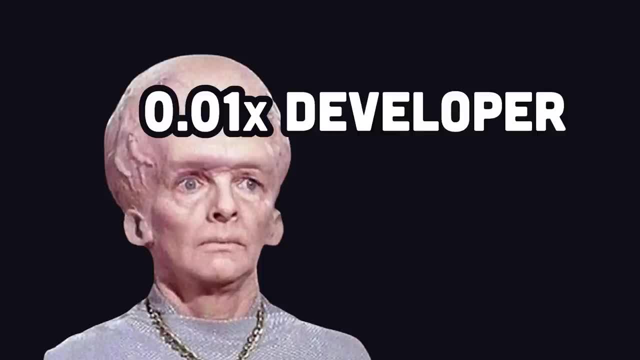 This allows search engines to display results properly and also helps with accessibility for devices like screen readers that allow anybody, regardless of disability, to enjoy the content. This allows search engines to display results properly and also helps with accessibility for devices like screen readers that allow anybody, regardless of disability, to enjoy the content. 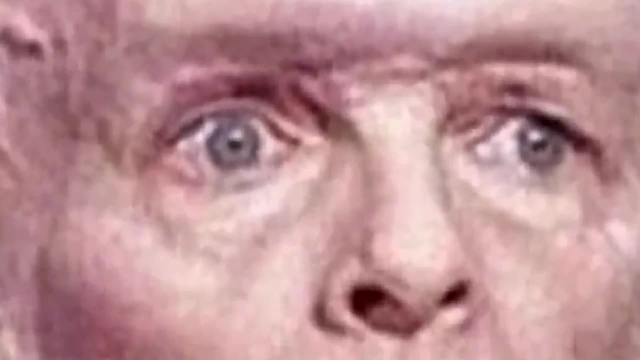 This allows search engines to display results properly and also helps with accessibility for devices like screen readers that allow anybody, regardless of disability, to enjoy the content. This allows search engines to display results properly and also helps with accessibility for devices like screen readers that allow anybody, regardless of disability, to enjoy the content. 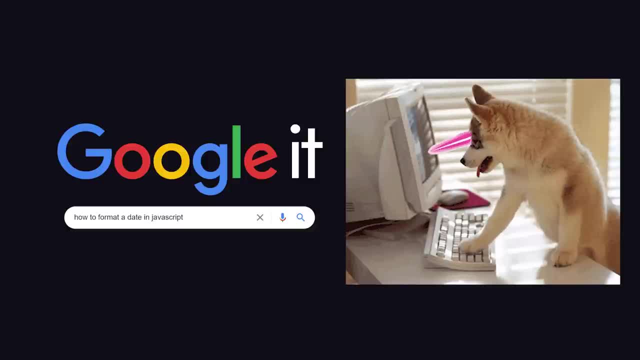 This allows search engines to display results properly and also helps with accessibility for devices like screen readers that allow anybody, regardless of disability, to enjoy the content. This allows search engines to display results properly and also helps with accessibility for devices like screen readers that allow anybody, regardless of disability, to enjoy the content. 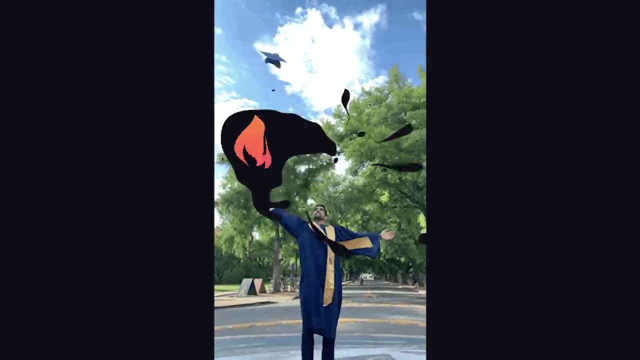 This allows search engines to display results properly and also helps with accessibility for devices like screen readers that allow anybody, regardless of disability, to enjoy the content. This allows search engines to display results properly and also helps with accessibility for devices like screen readers that allow anybody, regardless of disability, to enjoy the content. This allows search engines to display results properly and also helps with accessibility for devices like screen readers that allow anybody, regardless of disability, to enjoy the content. This allows search engines to display results properly and also helps with accessibility for devices like screen readers that allow anybody, regardless of disability, to enjoy the content.